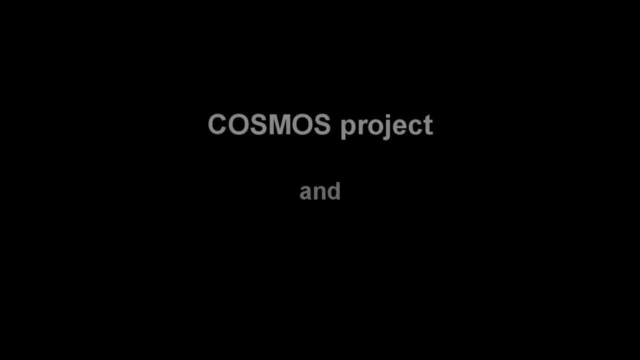 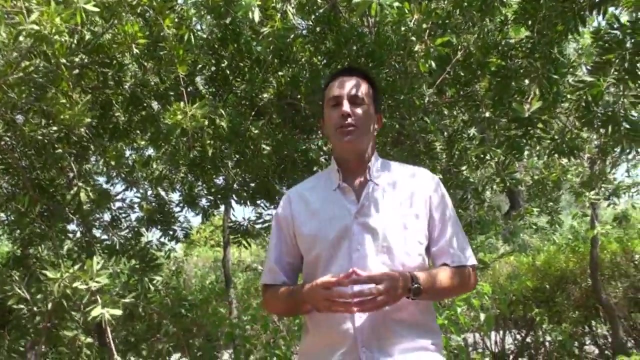 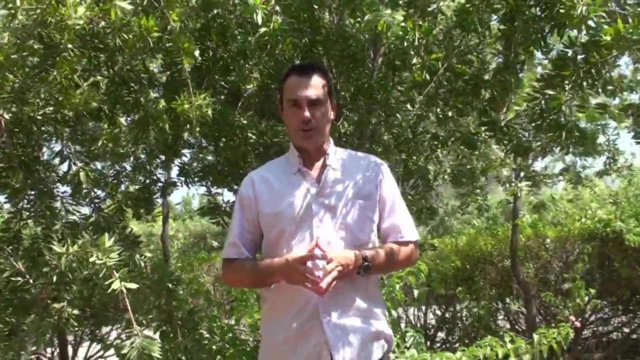 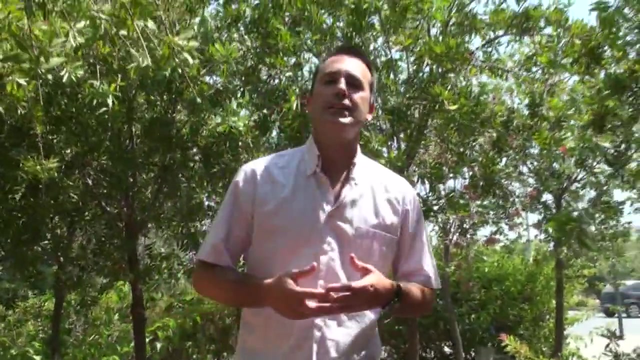 My name is Pablo Retz and I am a senior researcher at the Skinner-Katz Astronomical Observatory. My areas of professional expertise are observational astronomy and high energy astrophysics. This video is an introduction to the tutorial. Analysis of Astronomical Images. 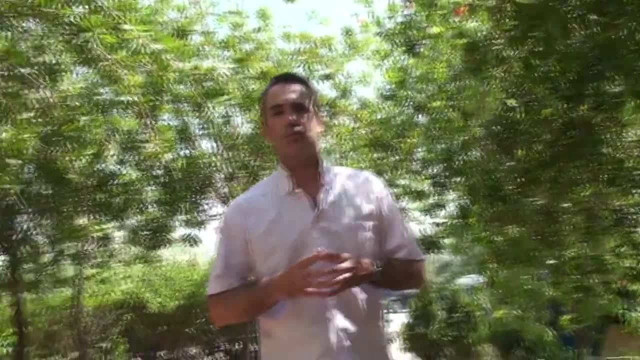 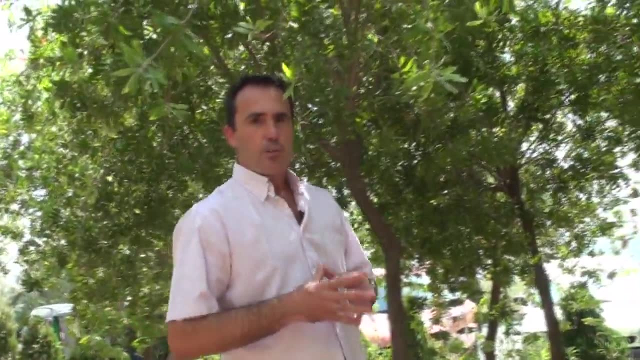 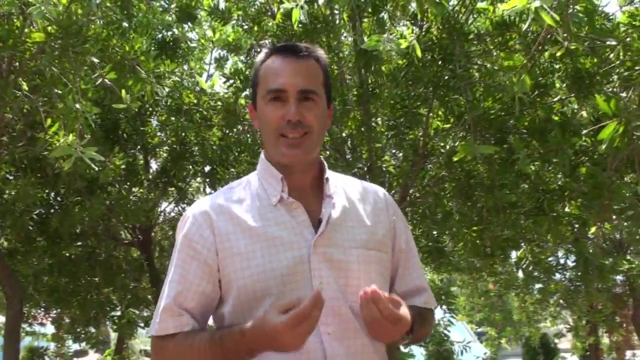 and explains the techniques that astronomers use in our days to photograph the sky. We will talk about CCD cameras, how to process a CCD image and how to assess the quality of an image by measuring the scene In the tutorial that follows this introduction. 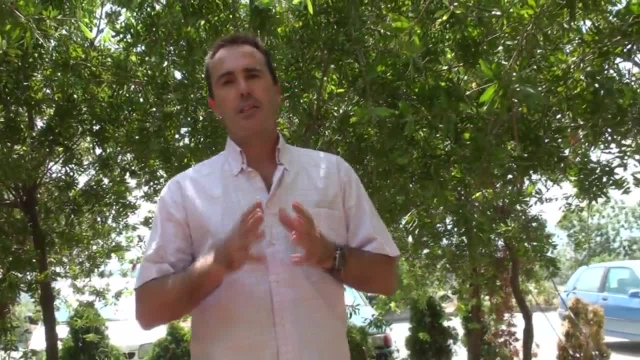 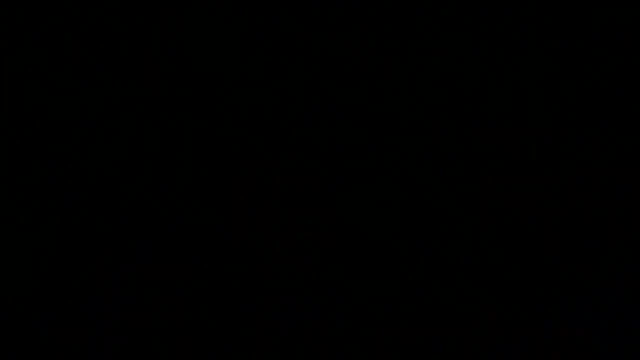 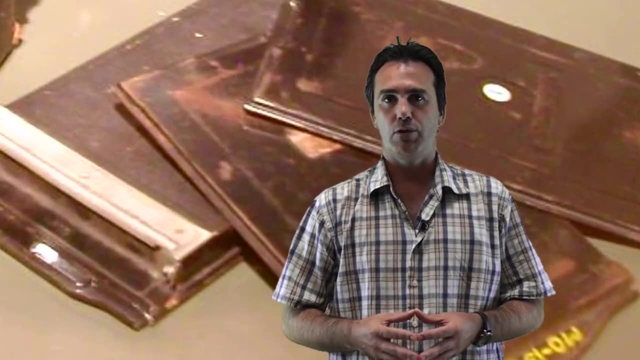 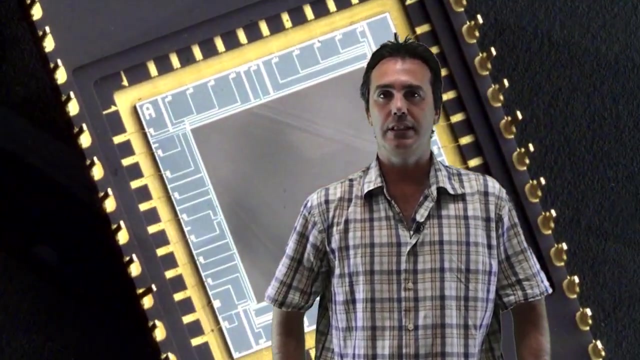 you will learn how to perform these tasks step by step, using dedicated software. Before the 70s and for more than 130 years, astronomers used photographic plates to take pictures of the sky. Nowadays they use electronic devices called CCD cameras. A CCD camera is an electronic instrument. 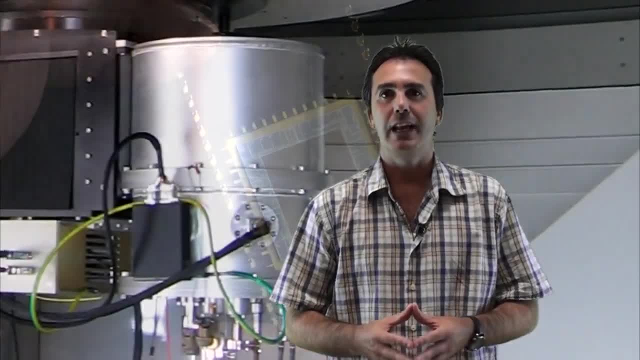 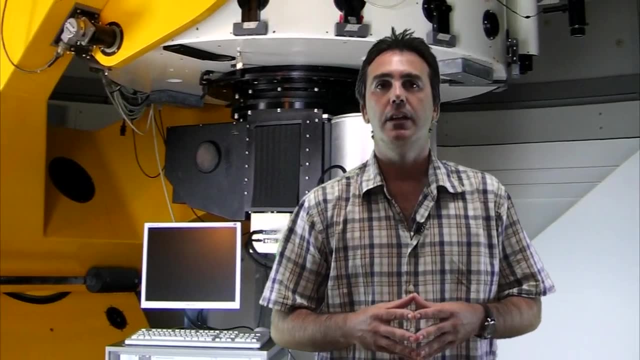 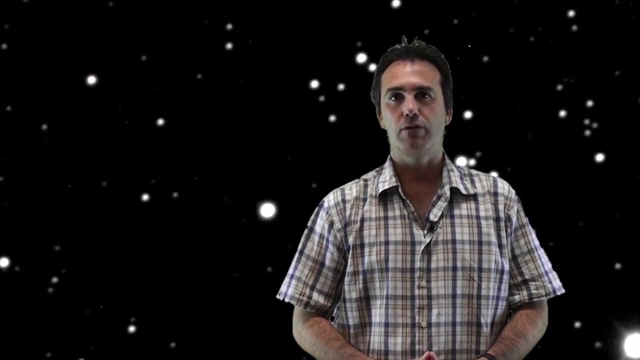 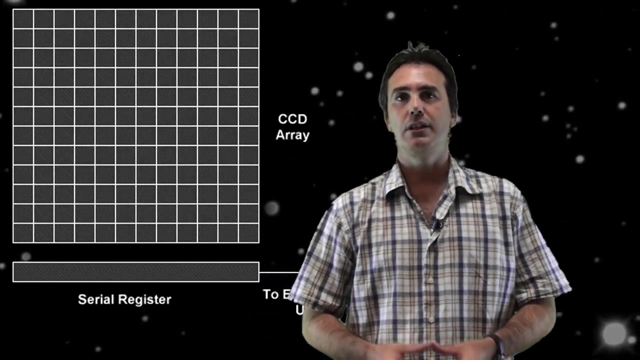 for detecting light In astronomy. the light coming from the stars is very dim, and this has certain implications for how the CCD operates. The acquisition of an electronic image is a relatively straightforward process. Photons of light strike a CCD image sensor and electrons are generated, collected and stored in individual cells or pixels. 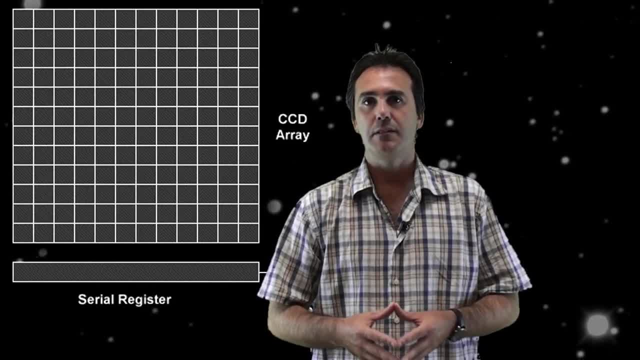 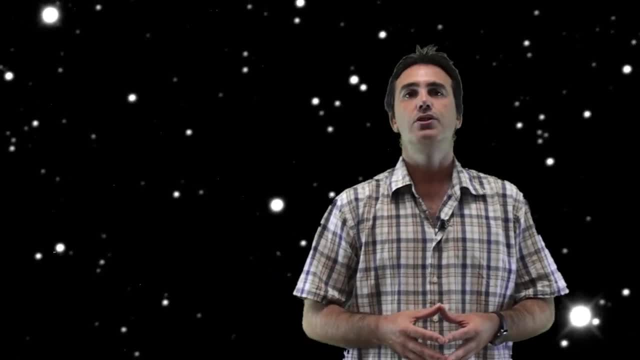 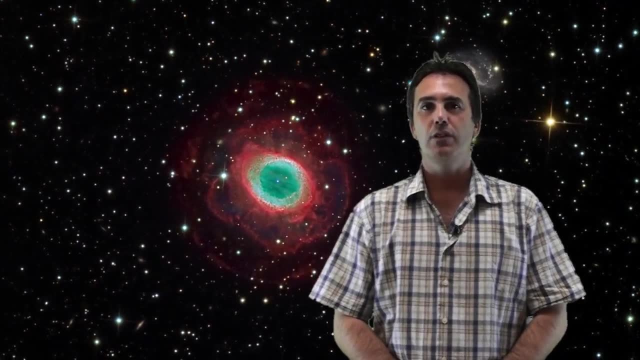 A numerical value is assigned to each pixel, based on the number of electrons contained in that pixel. This value is sent to the computer, which generates an image. Unfortunately, the image data that we collect and store does not contain only those electrons that truly represent light from the star. 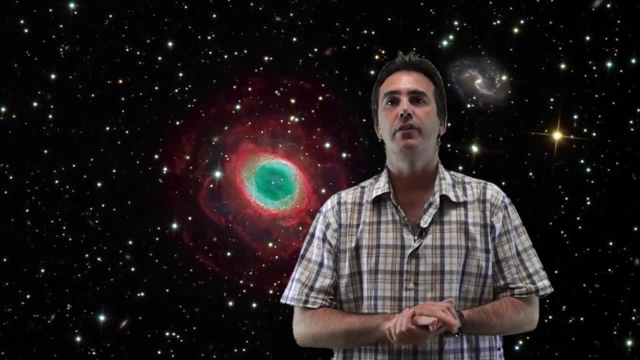 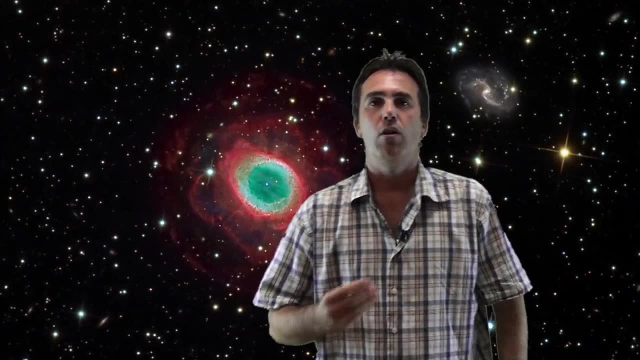 Imprinted on the raw image. there are a number of effects that are due to the nature of the detector and telescope and do not come from the object under study. All these instrumental artifacts have to be accounted for and removed, since they produce unwanted effects. 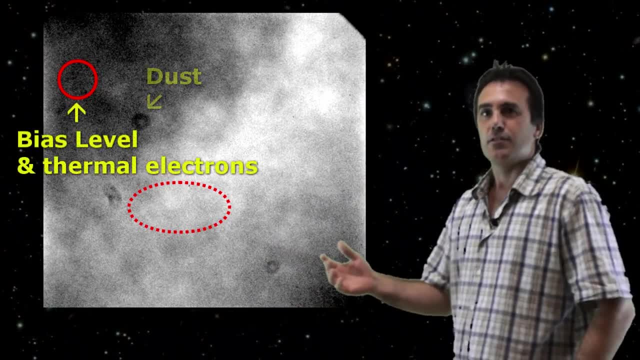 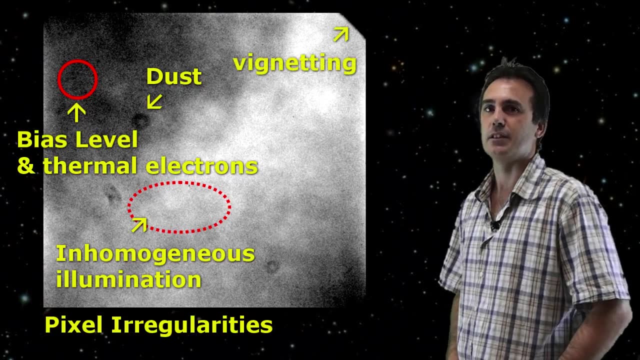 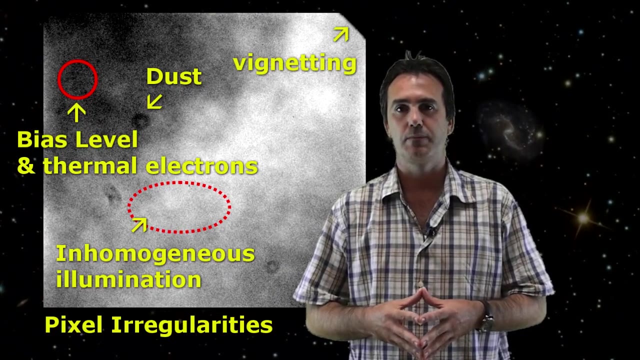 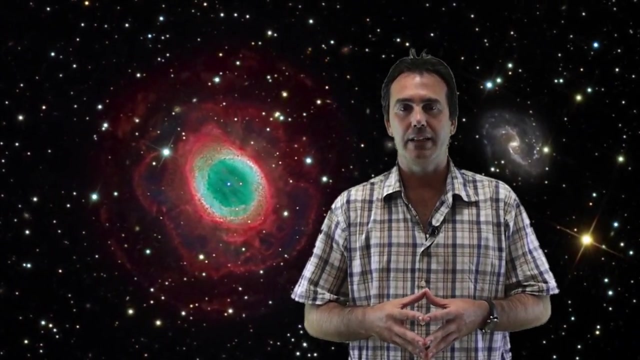 Thermal electrons, dust modes in homogeneous illumination, pixel irregularities, vignetting are some of these artifacts. Image processing software allows the removal of most of these artifacts. This video shows the basic steps of CCD image correction and cleaning, including the use of calibration frames. 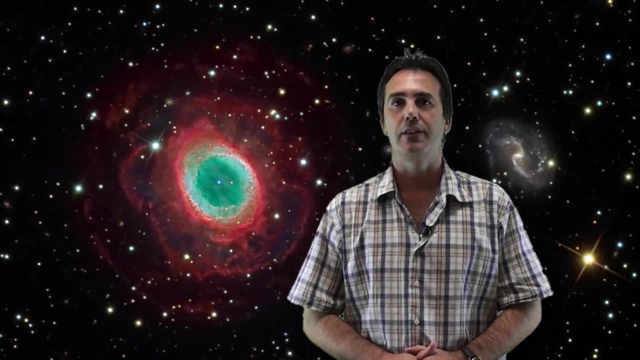 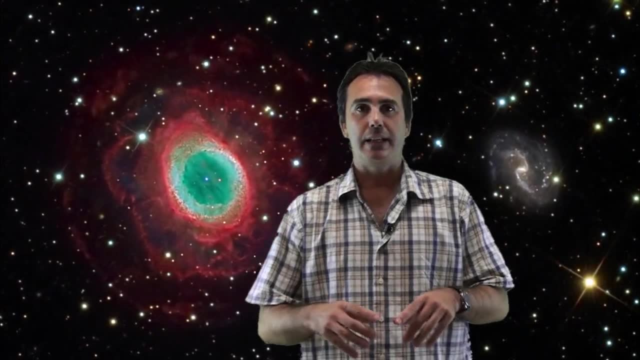 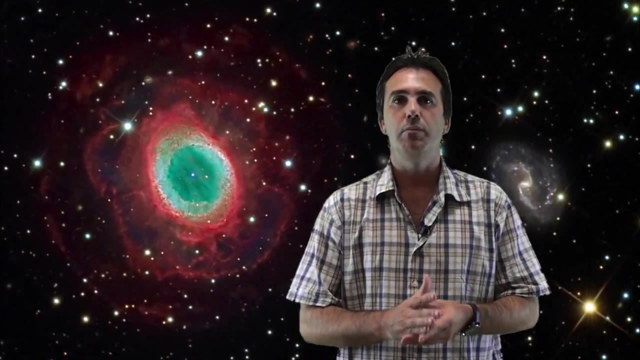 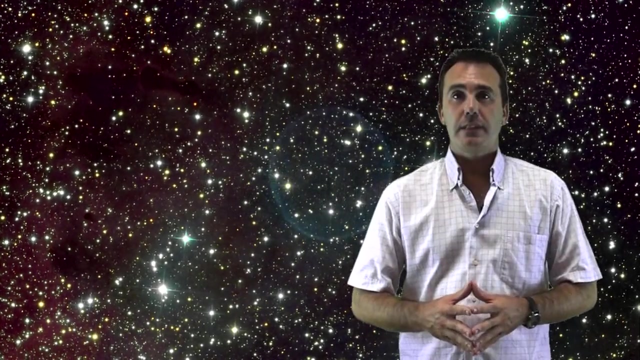 that correct the raw CCD image obtained at the telescope so that scientifically meaningful data can be extracted. In the tutorial Analysis of Astronomical Images that accompany this video, each one of these steps will be performed using real observations. In astronomy, seeing refers to the clarity. 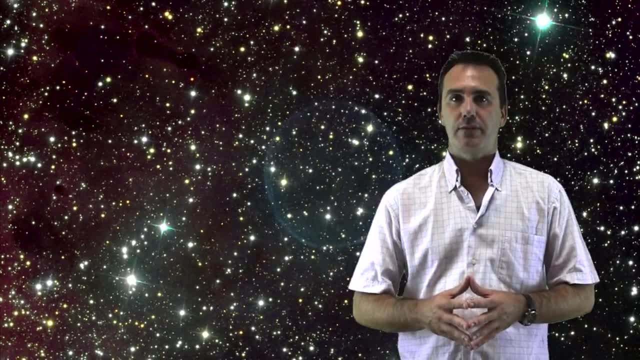 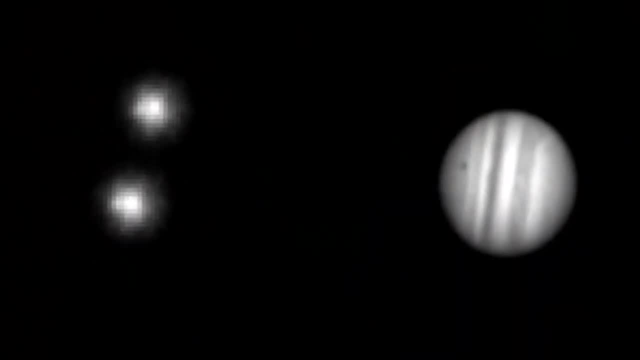 with which stars and other celestial objects can be observed. It is primarily determined by the atmosphere of the Earth. The most obvious phenomenon is twinkling, when the brightness of a star seems to fluctuate. The most common scene measurement is the diameter of the point spread function. 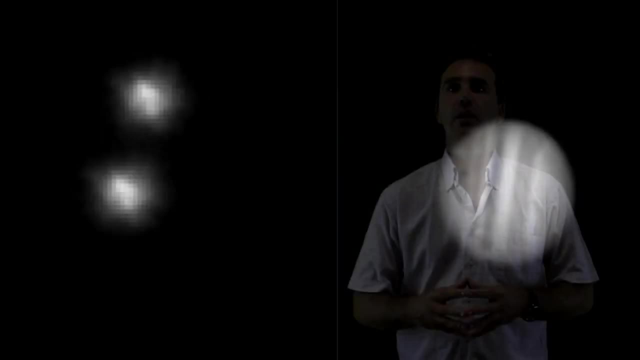 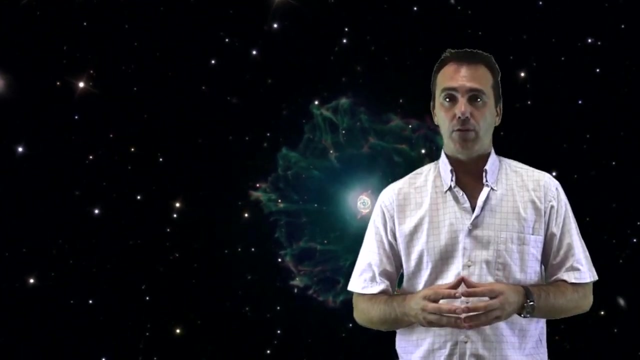 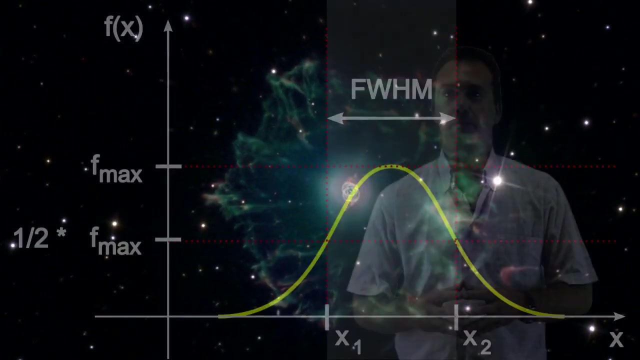 The point spread function diameter gives the best possible angular resolution which can be achieved by an optical telescope in a long exposure and corresponds to the diameter of the fuzzy blob seen when observing a point-like star through the atmosphere. The scene is estimated by measuring the full width. 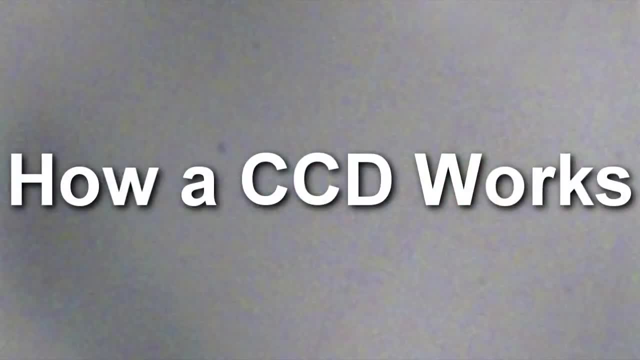 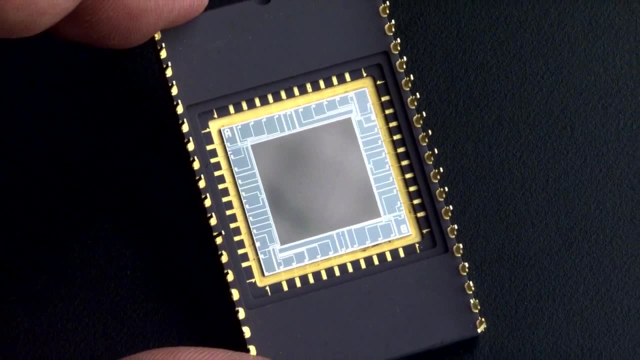 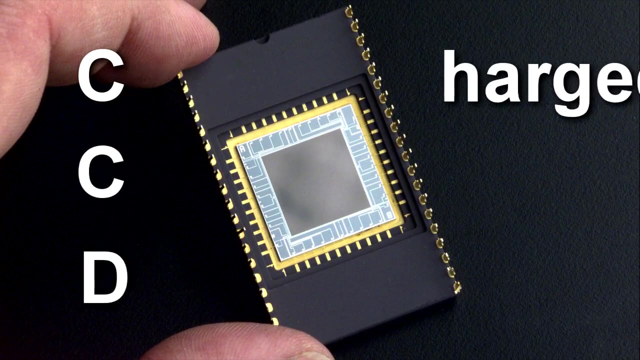 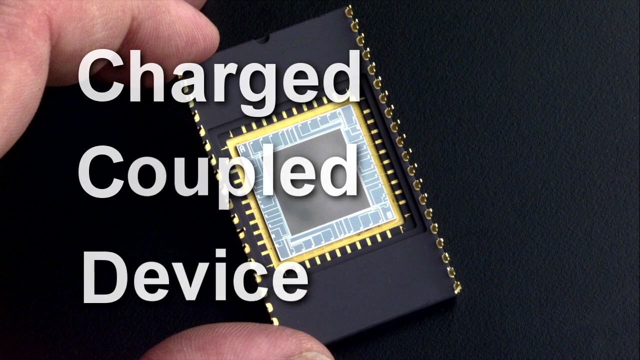 at half-maximum of the point spread factor. First, let's see in more detail how a CCD operates. CCD camera is an electronic instrument for detecting light. CCD stands for Charge Copied Device and consists of a semiconductor chip, one phase of which is sensitive to light. 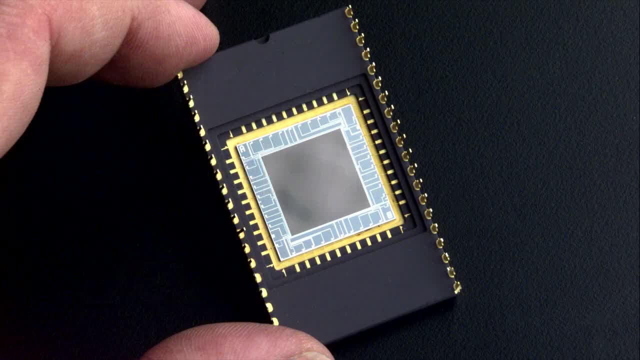 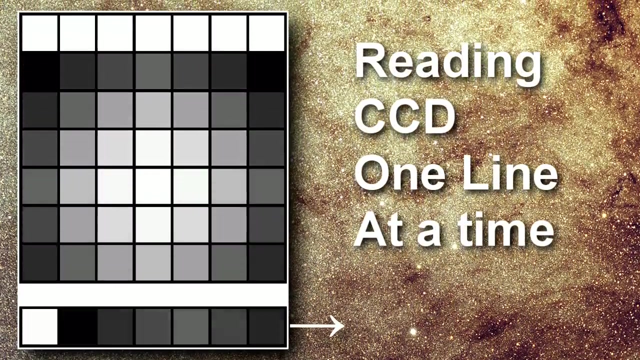 The CCD chip plays a similar role to the film of a traditional camera. The light-sensitive phase is rectangular in shape and subdivided into a grid of discrete rectangular areas known as picture elements or pixels. The arrival of a photon on a pixel generates a small electrical charge. 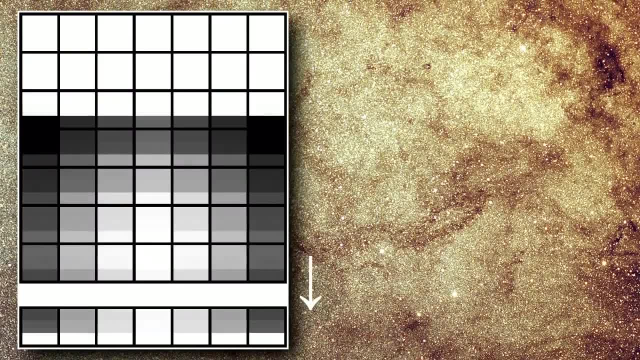 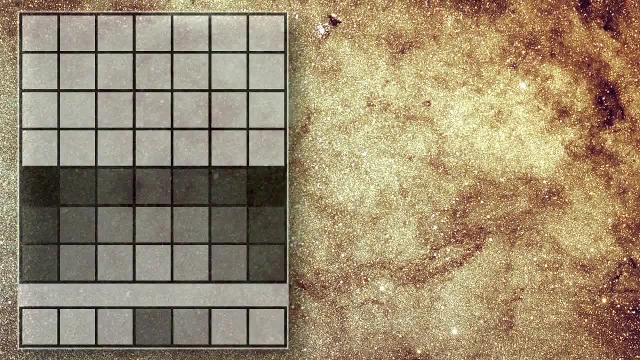 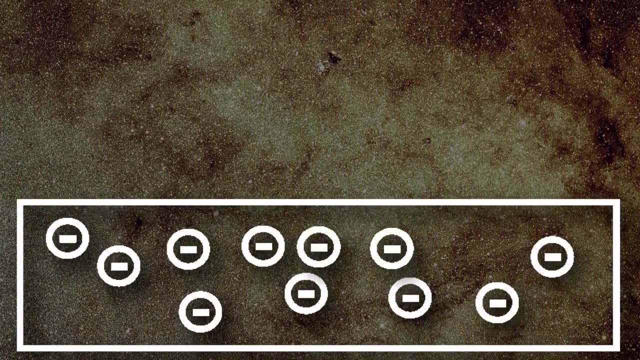 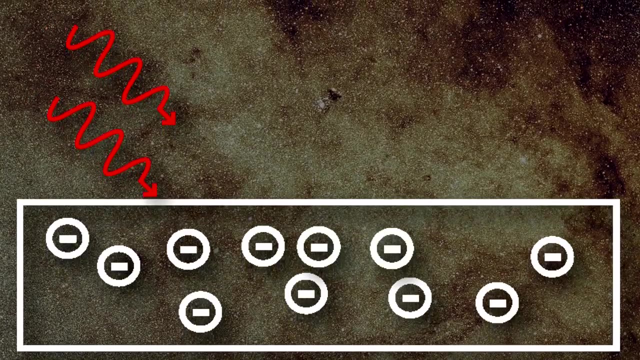 The size of the charge increases as more photons strike the surface, The brighter the illumination, the greater the charge. Charge is generated through the photoelectric effect. The photoelectric effect is the process in which electrons are emitted from the surface of a metal in response to incident light. 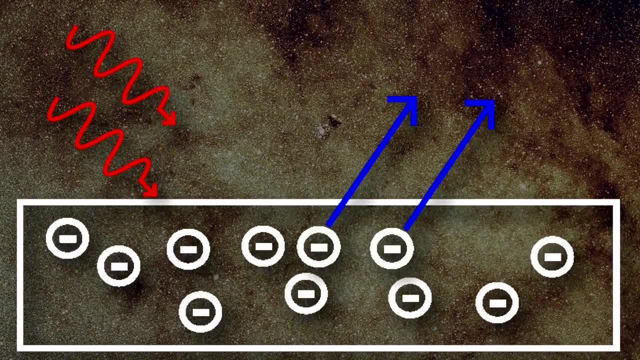 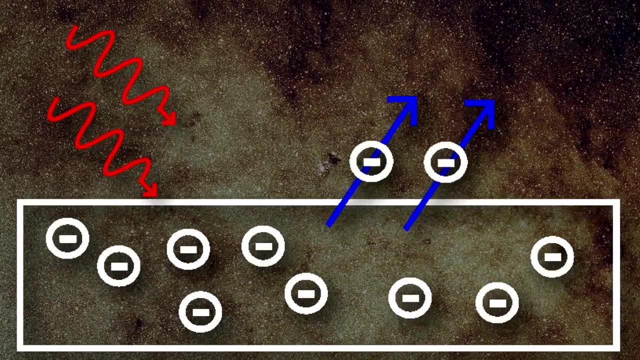 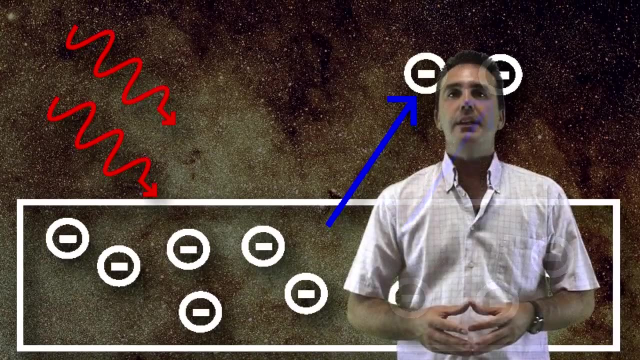 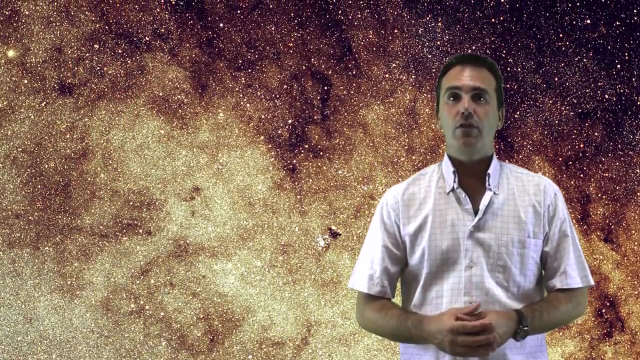 The energy of the incoming photon is absorbed by the electrons, giving them enough energy to be emitted from the surface of the metal. The emitted electrons are referred to as photoelectrons. Individual charge packets are converted into an output voltage. The output voltage is converted to a digital number. 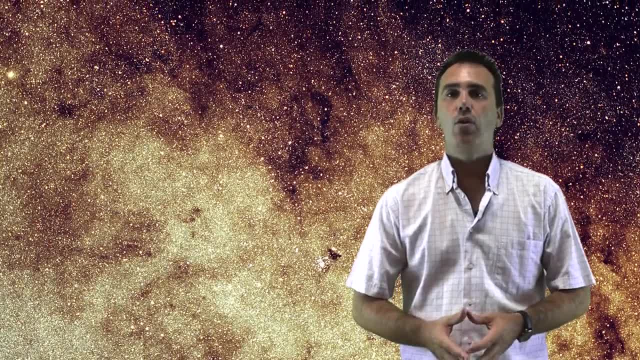 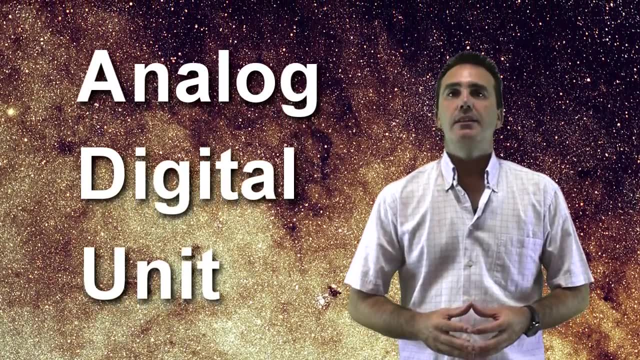 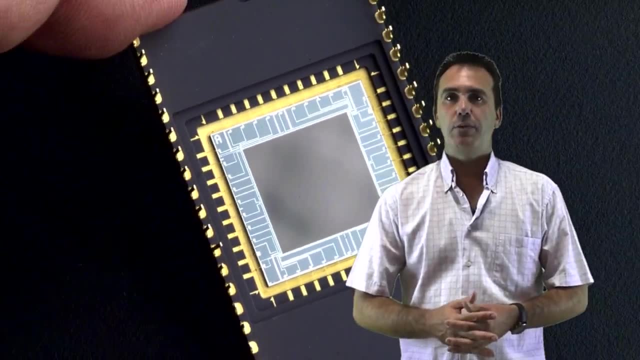 known as counts or ADU, analog to digital units. The size of a pixel is typically 10 to 30 microns across. Modern CCD chips have between 2,000 and 4,000 pixels, which means that the dimension of a CCD chip. 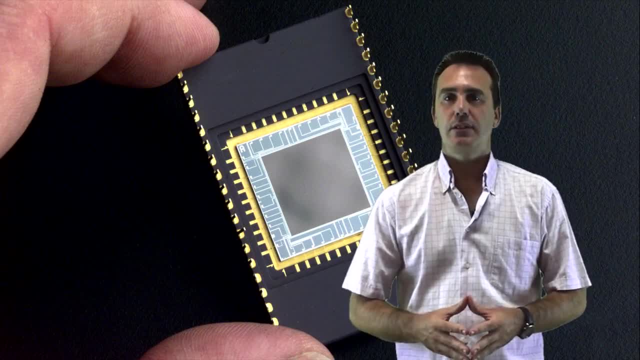 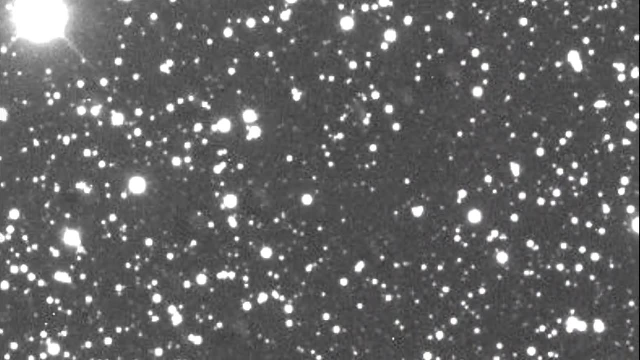 is typically between 1 to 3 centimetres on each side. The pixel size of a pixel is typically between 1 to 3 centimetres on each side. The pixels are so small that, in a typical situation, the image of a star may be spread out over several adjacent pixels. 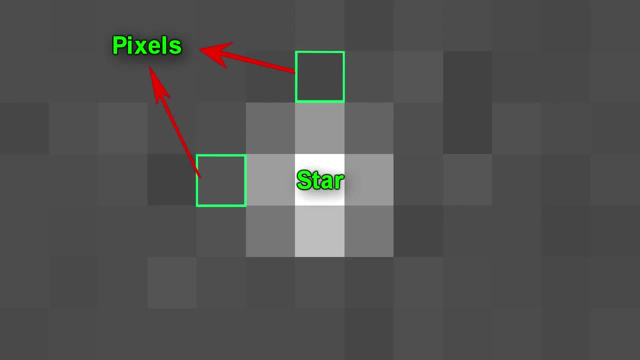 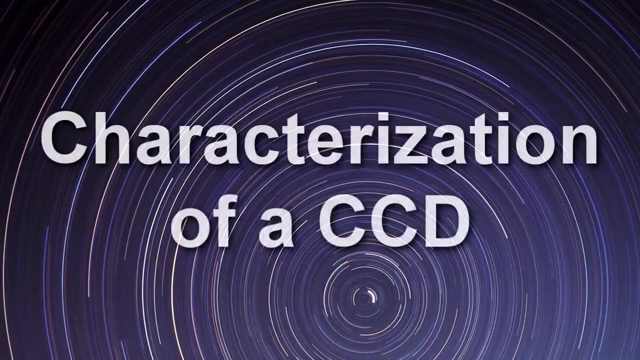 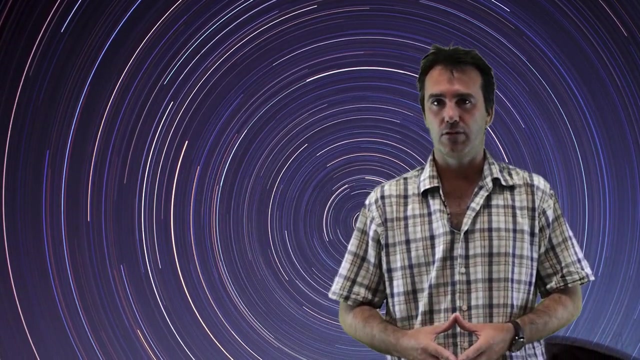 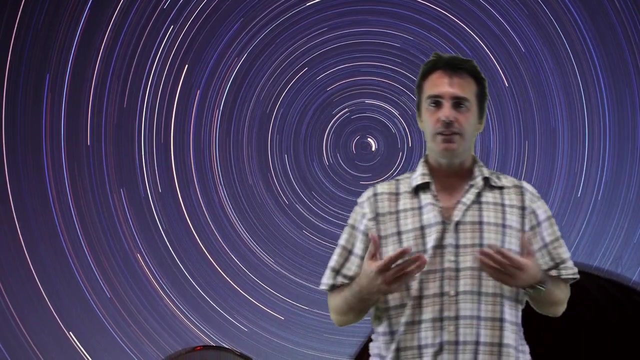 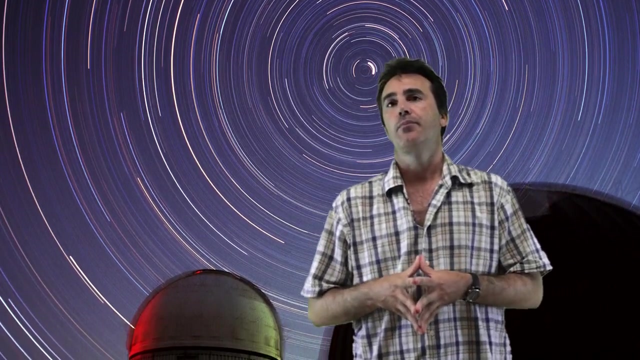 The more pixels, the greater the detail. There are a number of terms that characterize a CCD detector that you may have heard of but that you do not quite understand. Terms like gain, quantum efficiency, dynamical range, red noise- all these terms are associated with the use of CCDs. 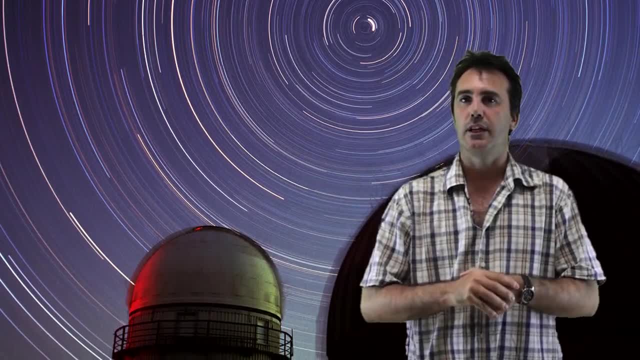 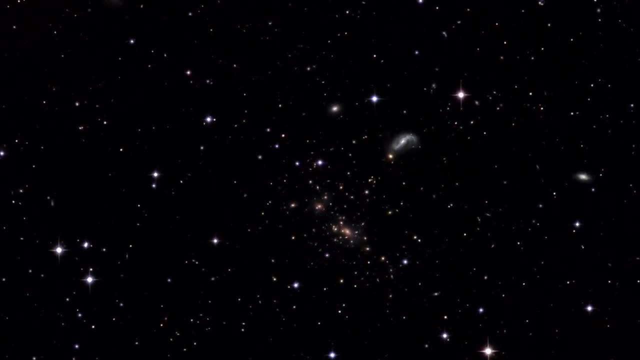 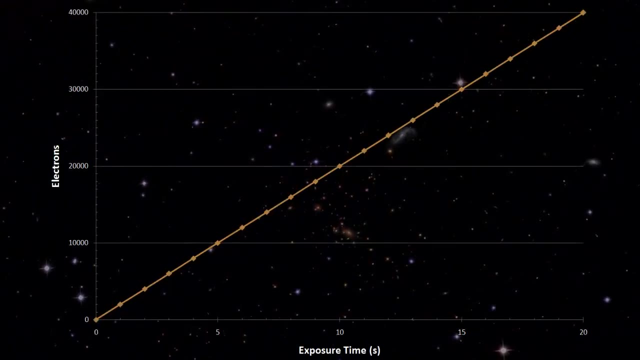 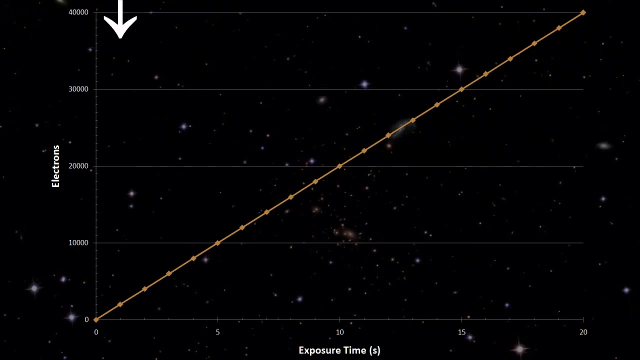 Let's now explain the meaning of these terms in more detail. One of the advantages of using CCD cameras with respect to photographic plates is linearity. Linearity is a measure of how consistently the CCD responds to light. For example, if a one-second exposure to a stable light source produces 2,000 electrons, 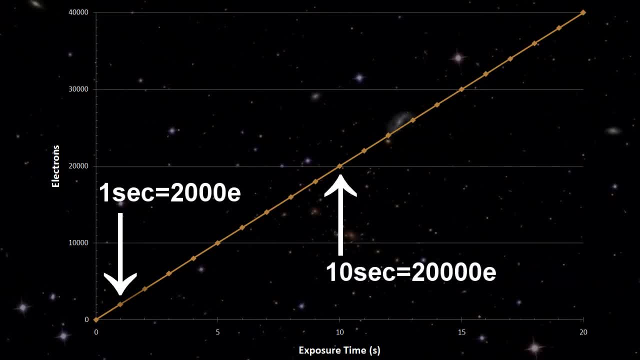 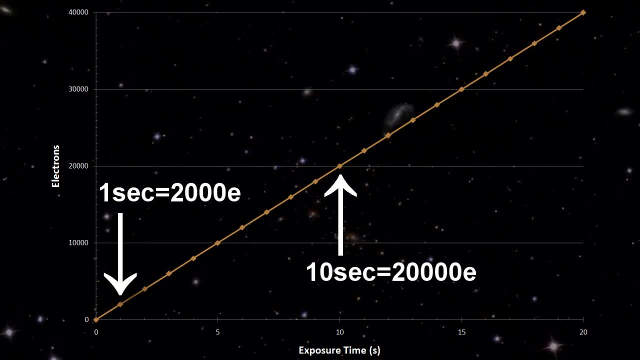 then a 10-second exposure should produce 20,000 electrons. In other words, there is a direct relationship between the intensity of the recorded image and the original exposure. Linearity also means that the number of electrons in a pixel is proportional to the number of incident photons. 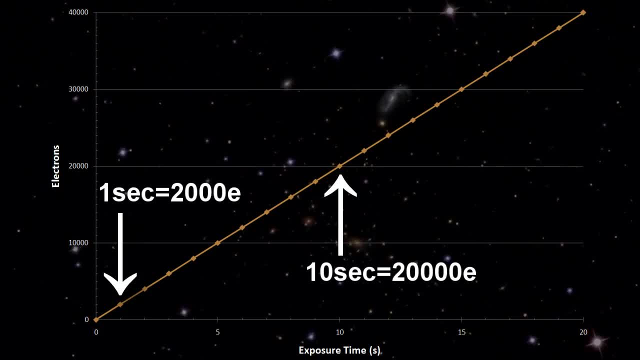 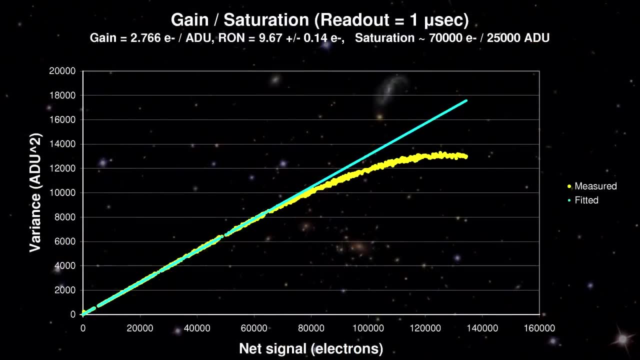 However, linearity is lost if the amount of incident photons is very large. Saturation and blooming are related phenomena that occur in all charge-coupled device image sensors under conditions in which the finite charge capacity of individual pixels is reached. Once saturation occurs, pixels lose their ability to accommodate additional charge. 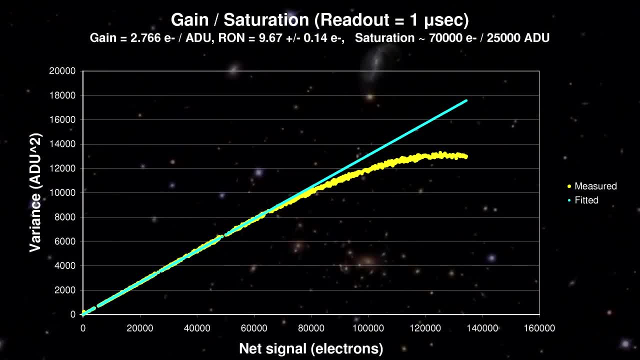 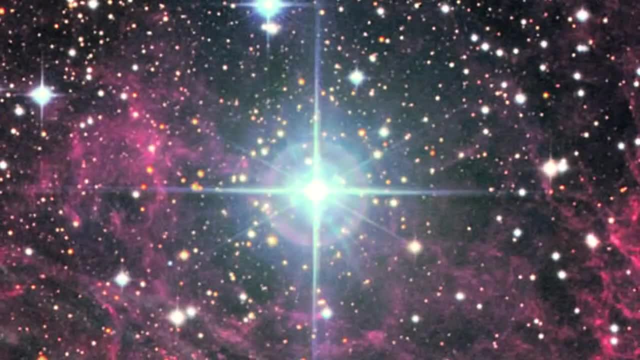 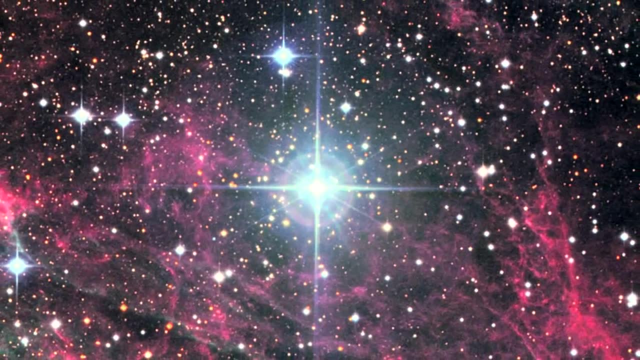 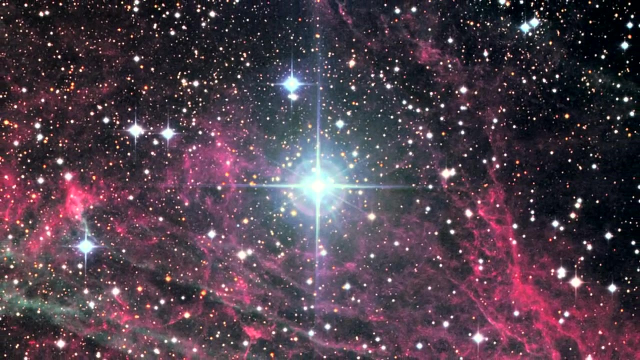 This additional charge will then spread into neighboring pixels, causing them to either report erroneous values or also saturate. This spread of charge to adjacent pixels is known as blooming and appears as a white streak or blob in the image. Each CCD has a different response and therefore the linearity range varies for different CCD cameras. 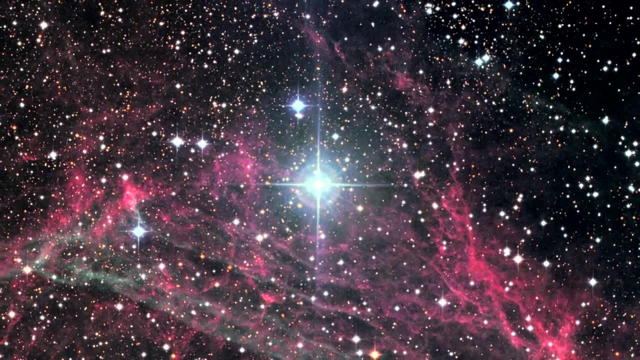 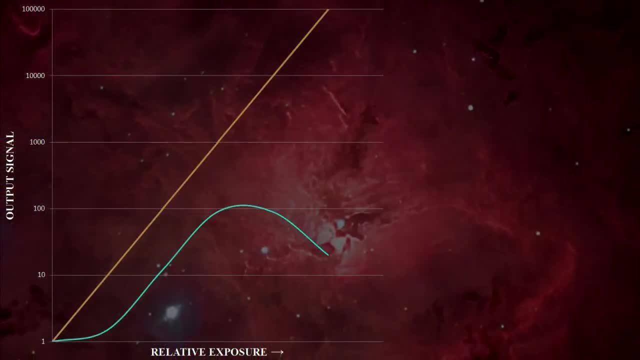 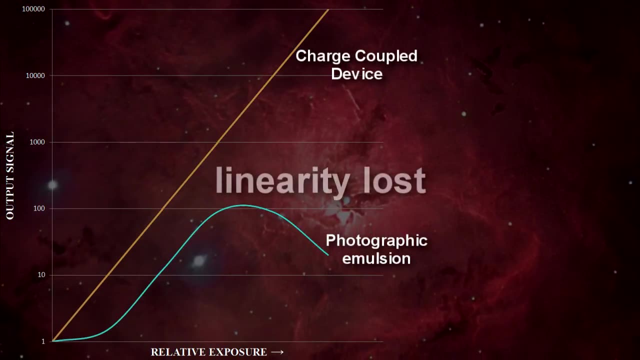 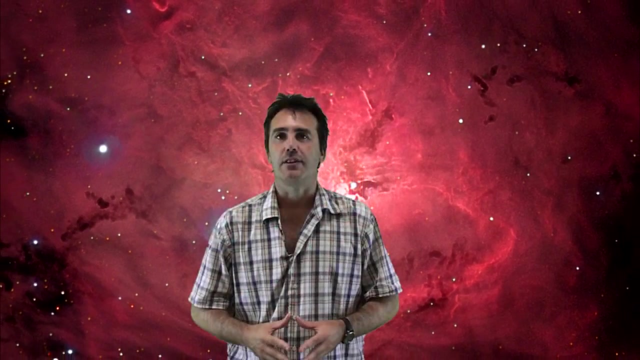 Deviations from linearity are often less than a few tenths of percent for over five orders of magnitude. This is far superior to photographic plates, which has a very limited linear regime. After the CCD chip has been exposed to light, the charge accumulated by each pixel. 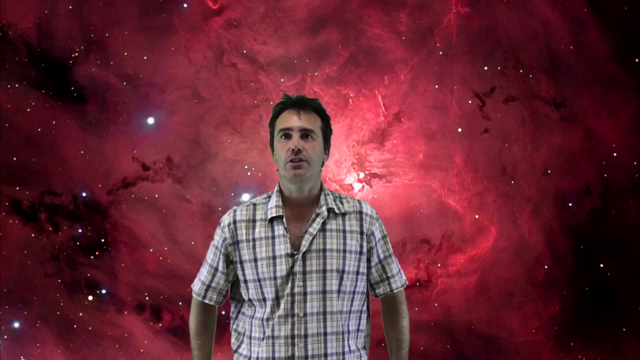 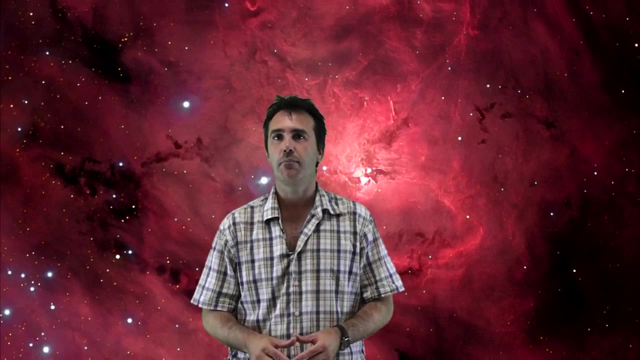 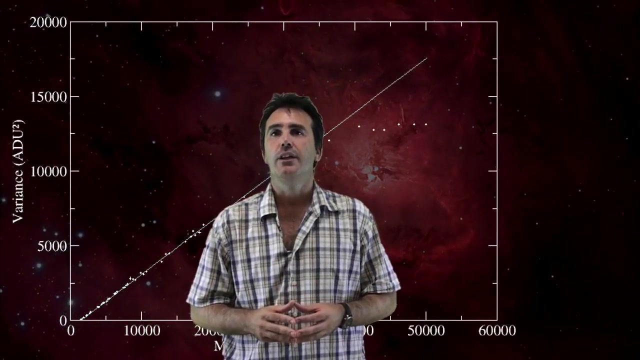 is read out. Individual charge packets are converted into an output voltage. The output voltage is converted to a digital number known as counts or analog to digital units. This value does not equate to the actual number of electrons detected in the pixel, but it is proportional to it. 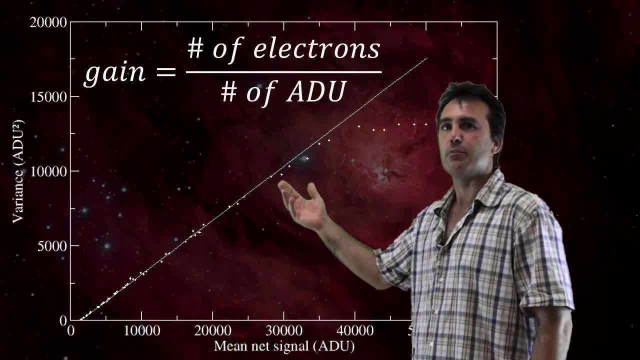 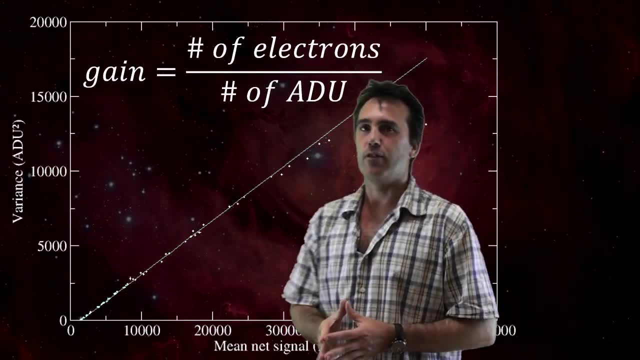 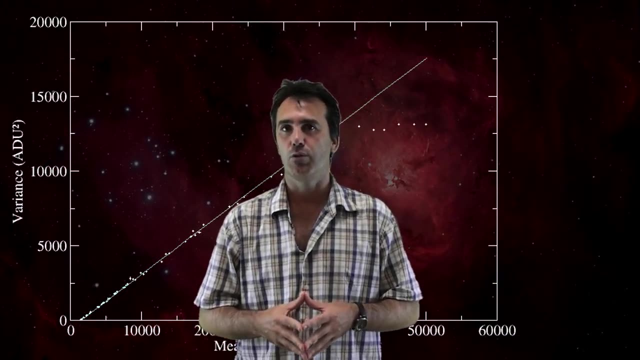 The number of collected electrons compared to the number of ADU is called the gain of the CCD. For example, a gain of 10 electrons per ADU means that for every 10 electrons collected in a pixel, the output voltage produces on average 1 ADU. 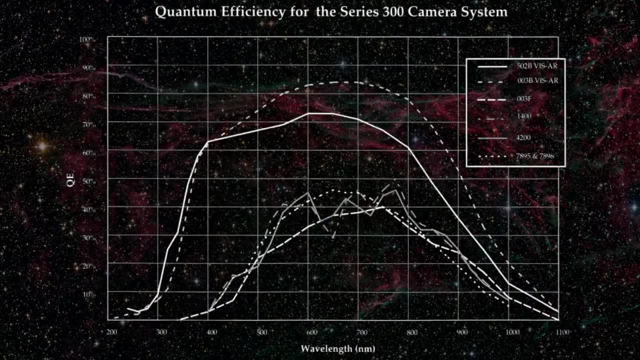 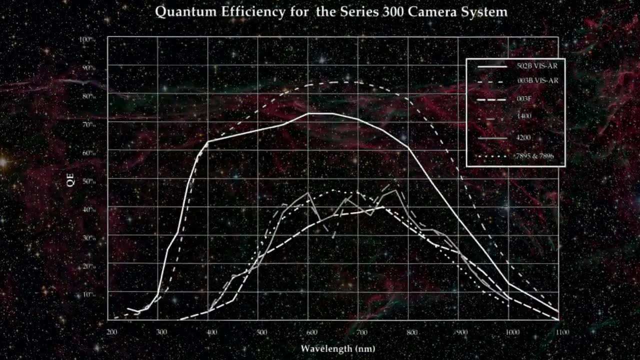 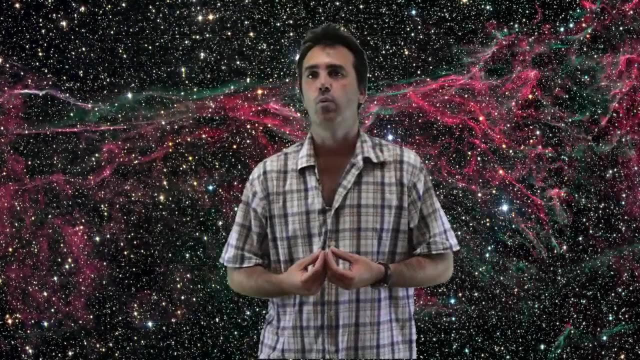 Quantum efficiency is the number of photoelectrons that are generated in a pixel for every photon of light that hits the surface above it. Quantum efficiency is, in simple terms, the percentage of light detected by your CCD. The quantum efficiency of a typical CCD camera is 90%. 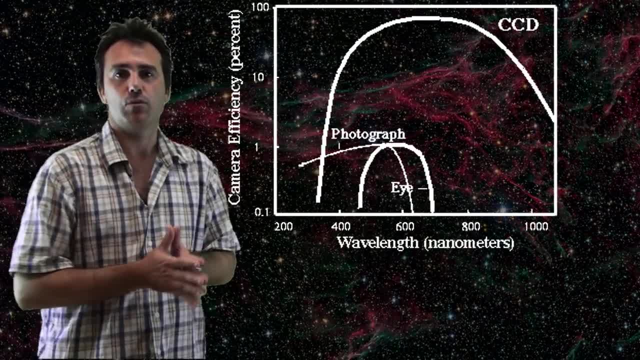 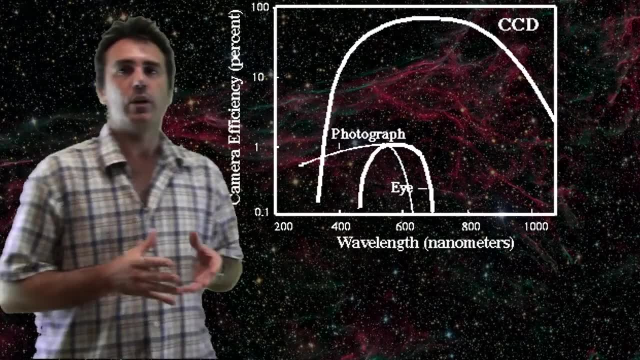 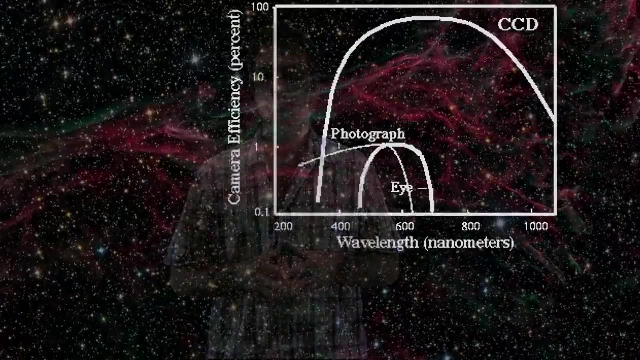 This value compares to just 1%, which is the typical quantum efficiency of a photographic plate. Putting a CCD camera on a 1-meter telescope gives it the same capability of a 4-meter telescope with a photographic plate. 3. Redout noise. 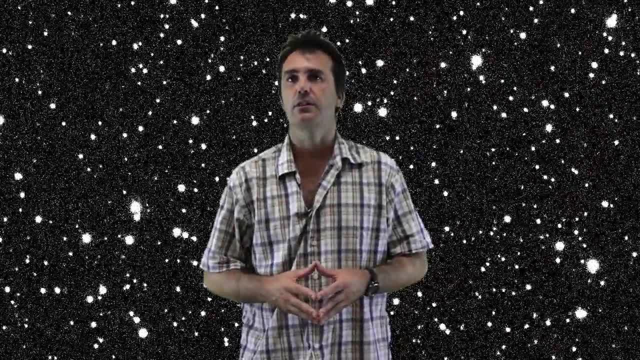 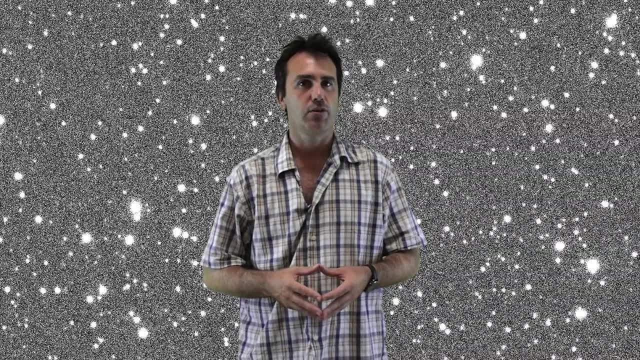 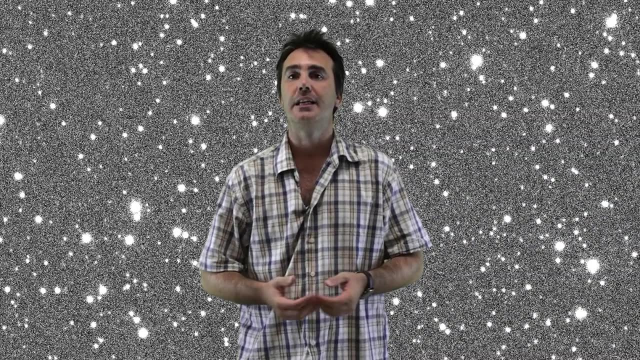 Redout noise, not just red noise, is the number of electrons introduced per pixel into the final signal upon redout of the device. Red noise is due to the uncertainty introduced by the amplifiers that convert the electrons into a voltage. Typically, each redout has an uncertainty of between 1 to 10 electrons. 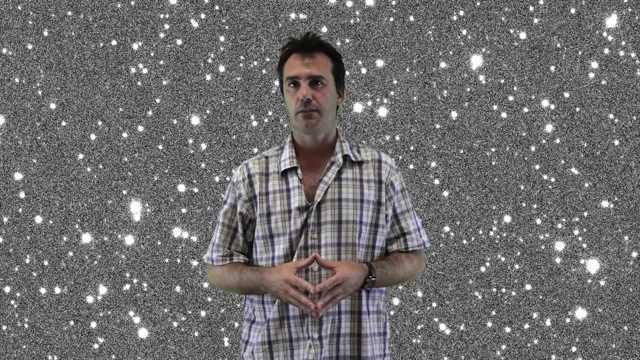 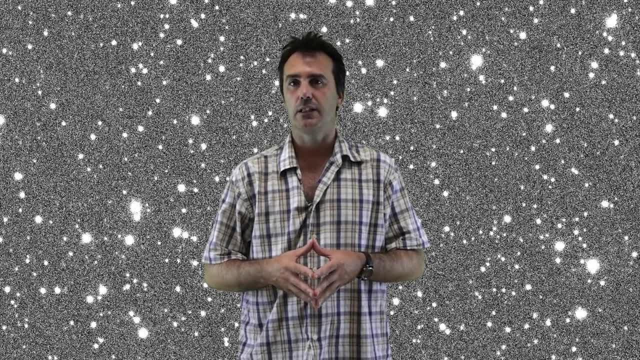 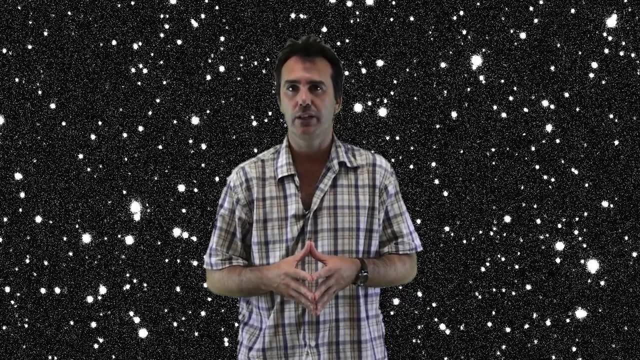 depending on the CCD and how it is operated. Red noise is one of the limitations on how faint an object a CCD can detect. In other words, the red-out noise places a limit on the magnitudes of the faintest stars which can be recorded. 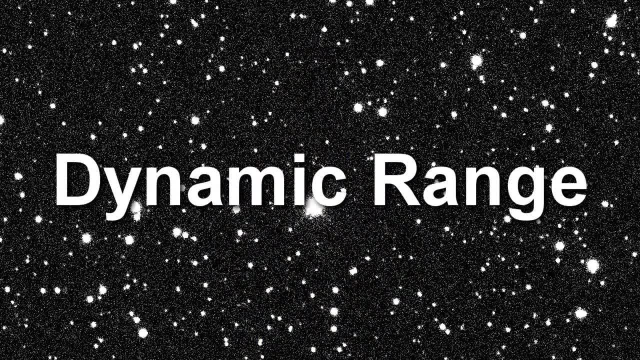 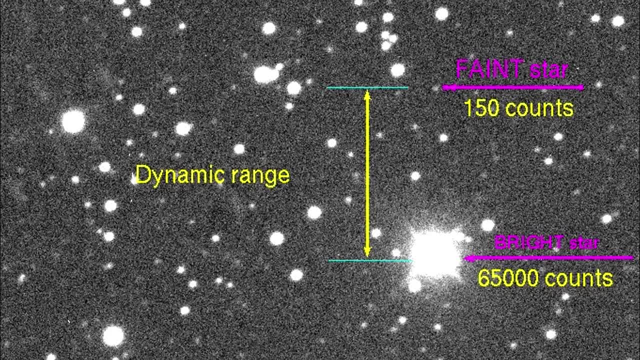 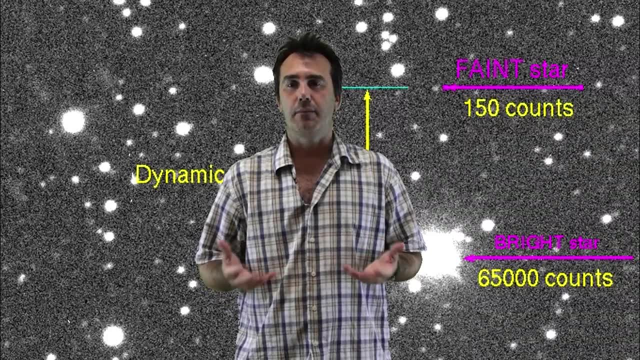 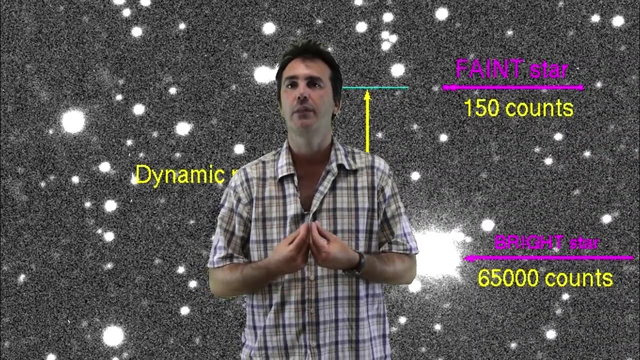 Dynamic range refers to the difference between the brightest and the faintest regions of an image that can be simultaneously recorded by the CCD camera. For a CCD camera, dynamic range can be estimated by dividing the full world capacity, that is the maximum number of electrons that a pixel can hold by the red noise. 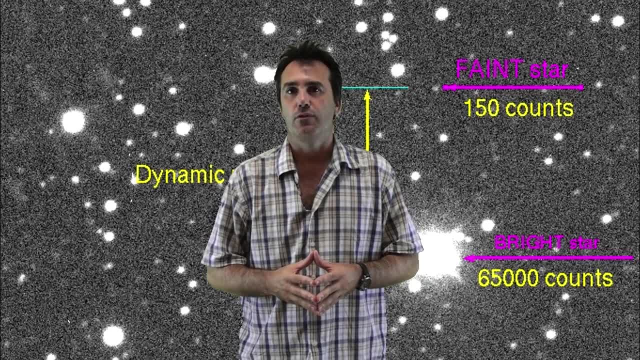 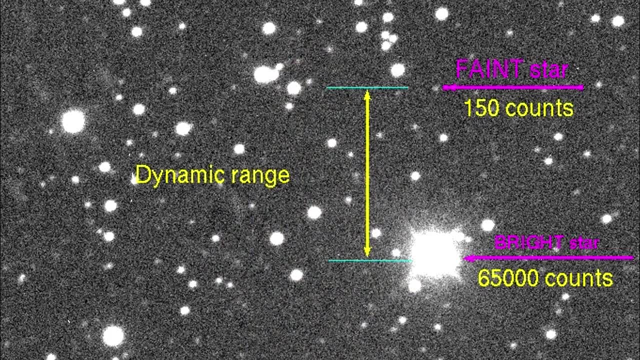 In other words by the red noise. The typical range for photographic materials may be of the order of 100 to 1.. In contrast, in CCD cameras it can be as large as 100,000 to 1.. That is, the dynamic range of a CCD camera is about 100 times larger compared to films. 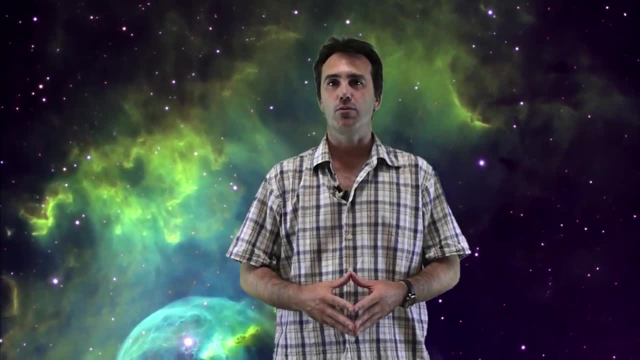 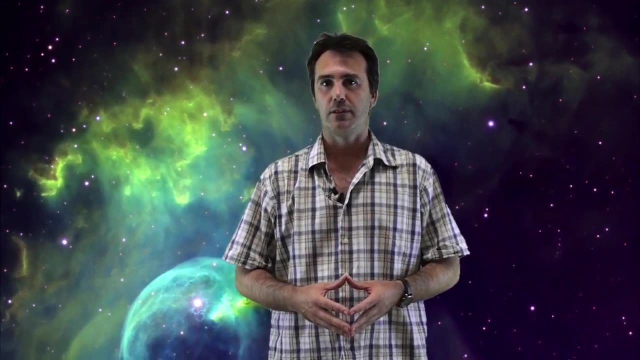 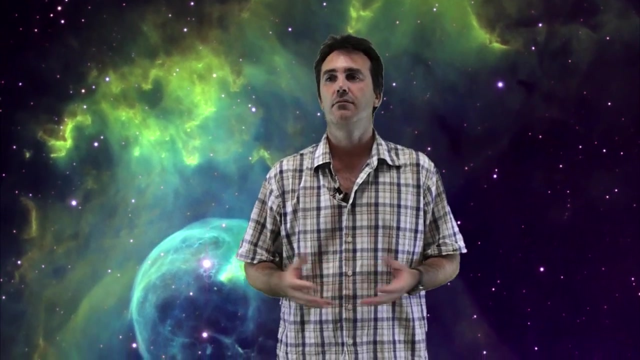 Current CCD cameras. Current CCD cameras have more than 60 million resolution elements or pixels. Image resolution is largely related to a characteristic of your system known as image scale, expressed as arcseconds per pixel. A low number for image scale, for example, 0.5 arcseconds per pixel. 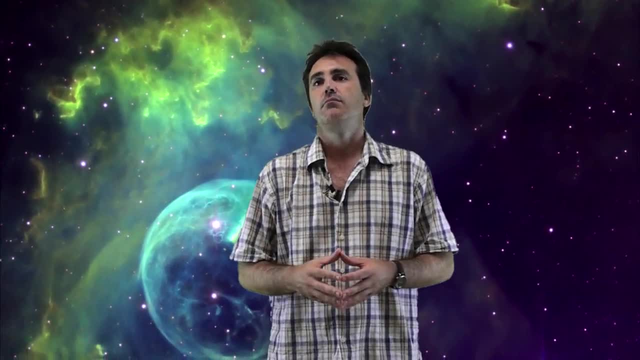 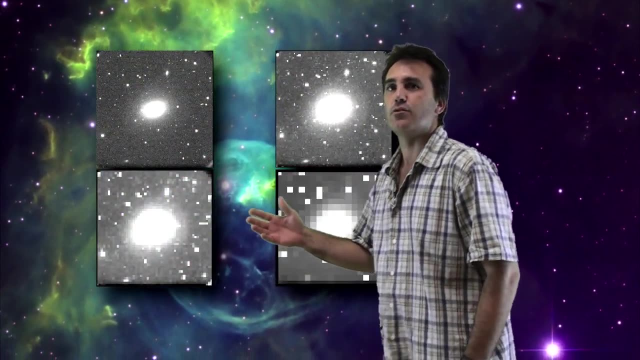 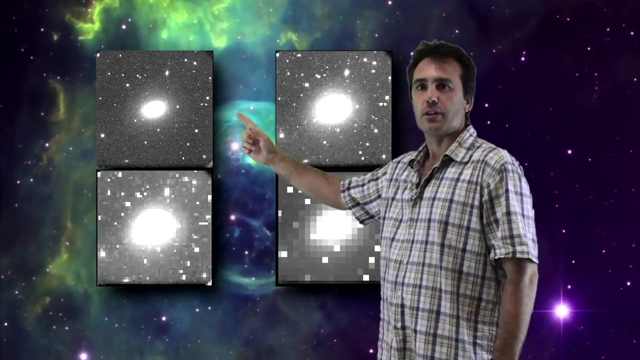 means high resolution, And a high number, let's say 10 arcseconds per pixel, means lower resolution. In this image you can see the loss of details when the spatial resolution is degraded. The image on the top left corresponds to the original image. 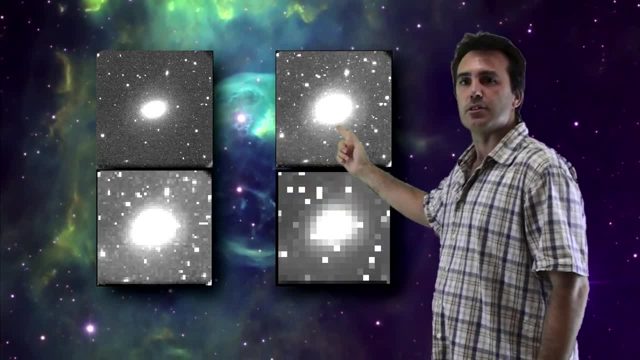 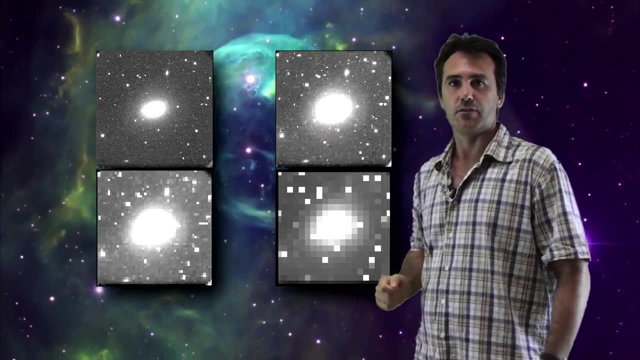 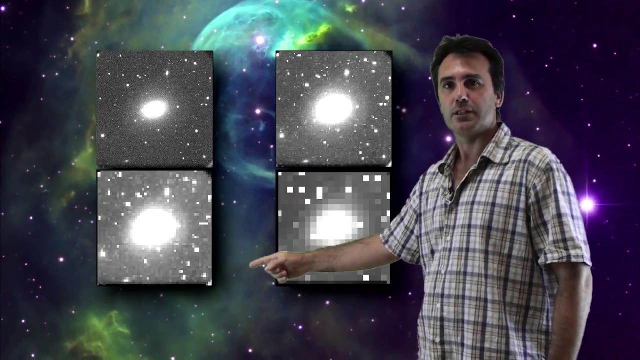 with full resolution. The image on the top right is the original image, re-beamed by a factor of 10.. That means that 10 pixels of the original image corresponds to 1 pixel. in this one, The image on the bottom left was re-beamed by a factor of 20,. 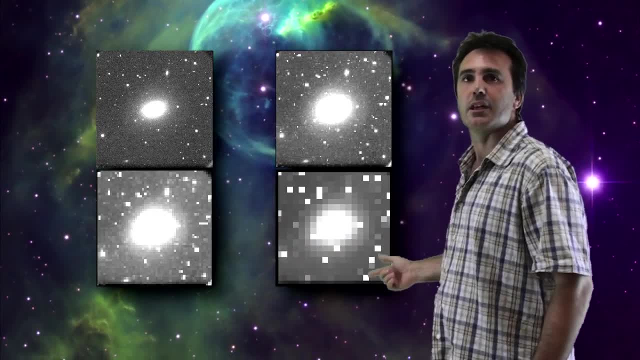 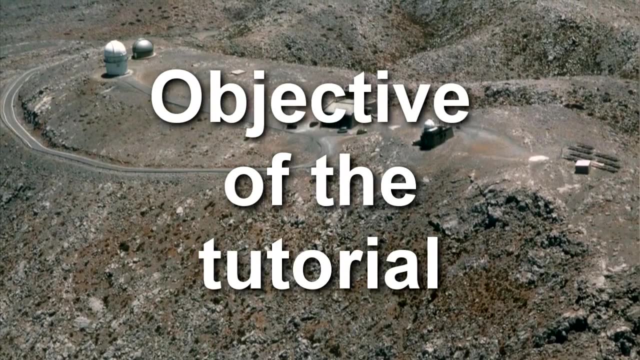 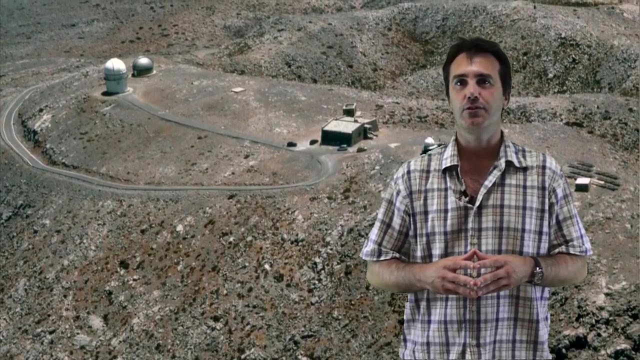 and the image on the bottom right corresponds to an image that has been re-beamed by a factor of 50.. Image resolution: As we mentioned before, the raw image, that is, the image obtained at the telescope, contains various instrumental artefacts that have to be removed. 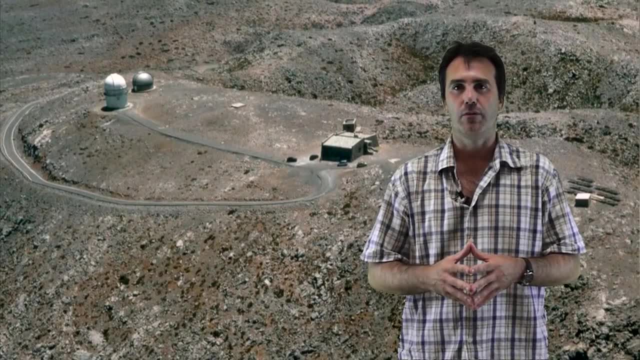 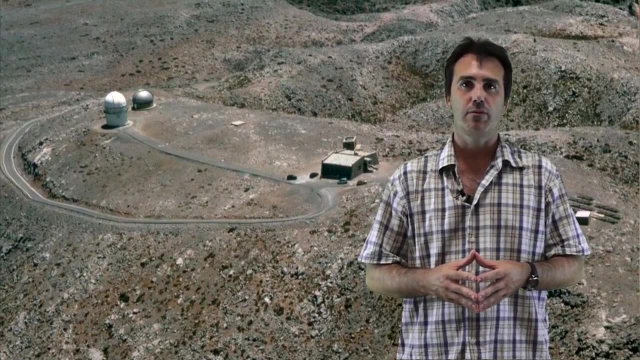 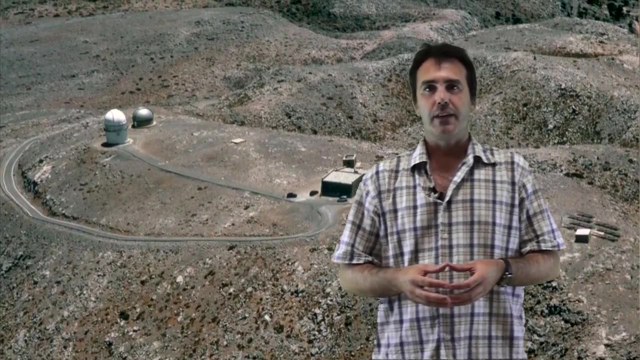 We will look into these effects in more detail now. In the tutorial Analysis of Astronomical Images that follows this video, you will learn how to perform all these necessary steps- necessary steps to clean and calibrate the raw image using real data. The artifacts commonly superimposed on data obtained with CCDs are either multiplicative: 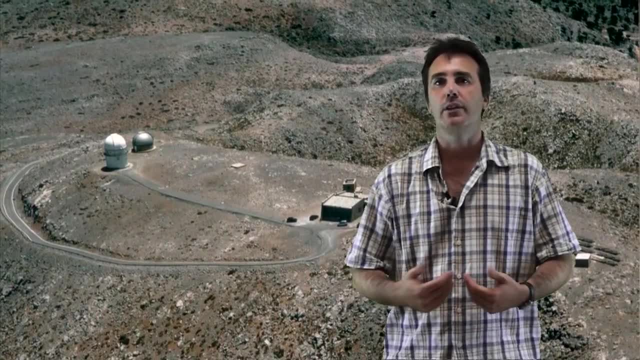 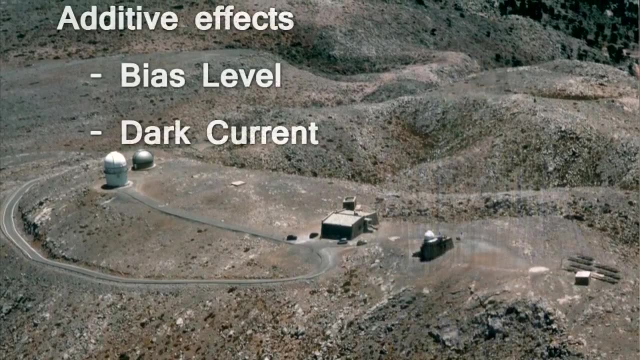 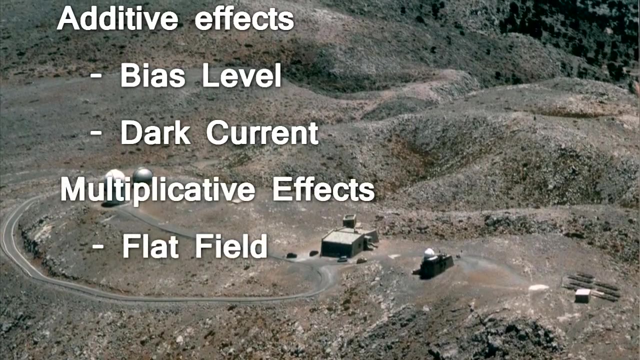 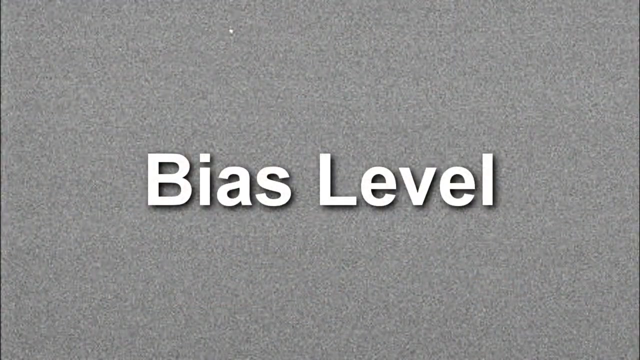 or additive. If they are multiplicative, one corrects for the error by division process. If they are additive, one corrects by subtraction. The two most important additive effects are electronic bias and thermal current. The most important multiplicative effect is pixel gain variation. 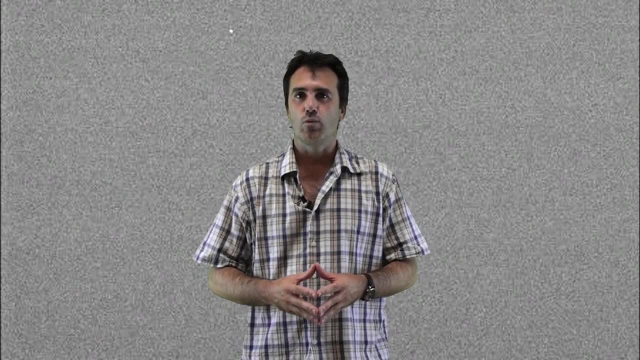 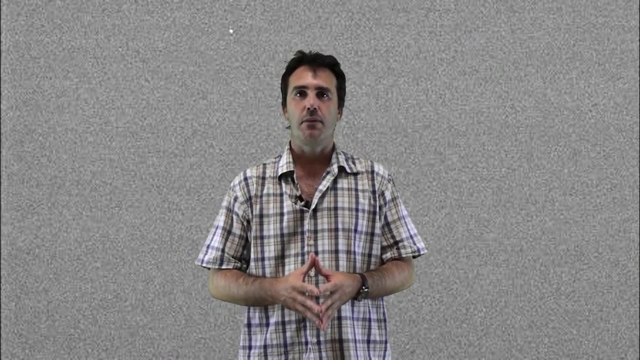 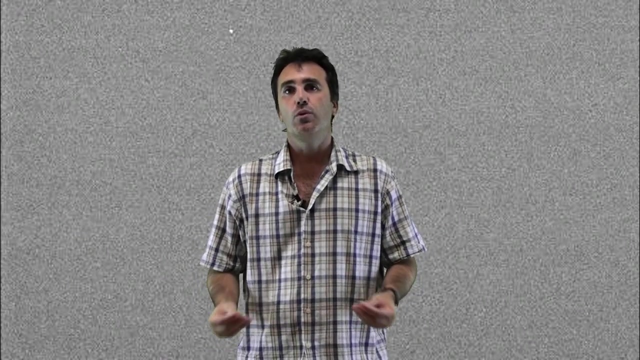 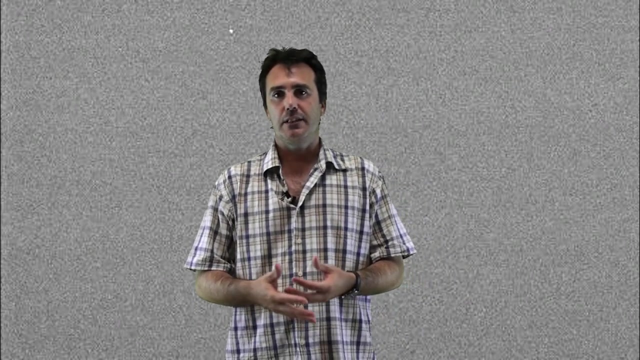 Bias level is an artificially induced electronic offset which ensures that the conversion from the accumulated charge to a digital value is positive. Bias frames are zero-second exposures obtained with the shutter closed. Therefore, we do not expect to see any start. The bias level is different in different CCD cameras. however, the bias value in a CCD 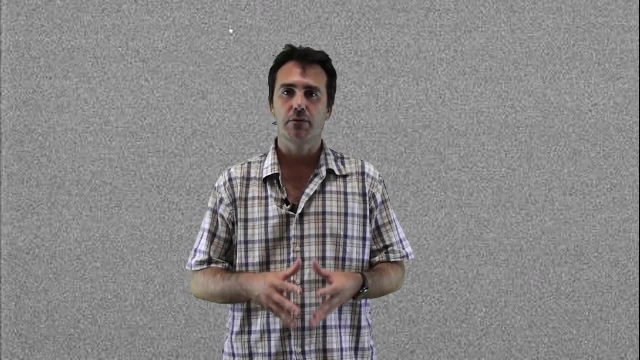 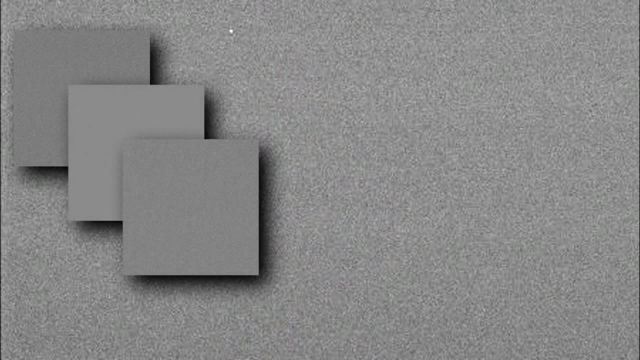 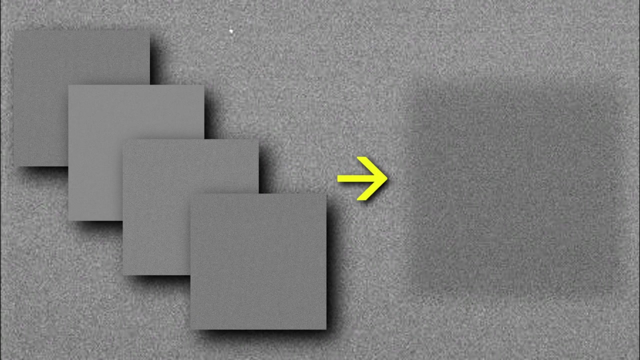 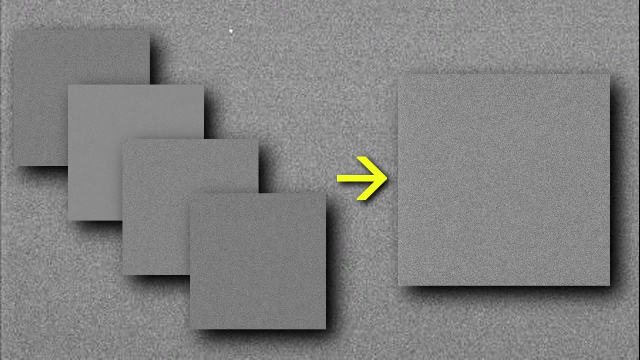 image is usually constant with time, except for statistical fluctuations. Single bias frame will not sample these fluctuations, so an average of 10 to 20 bias frames is recommended. The bias level is an additive effect. Therefore The mean bias frame has to be subtracted from all other images, data, frames and flat. 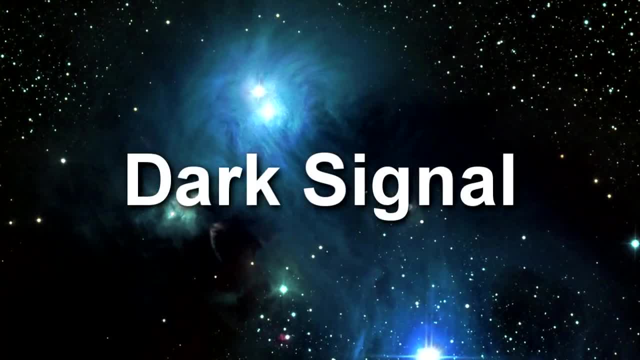 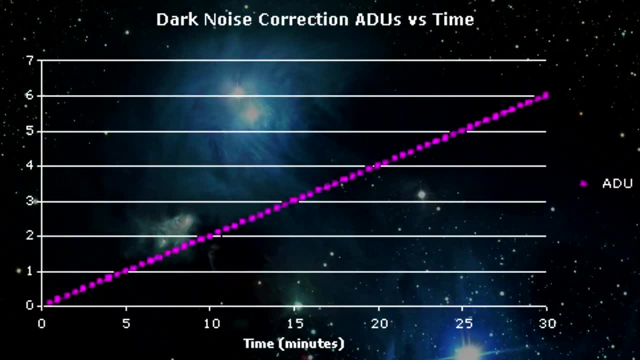 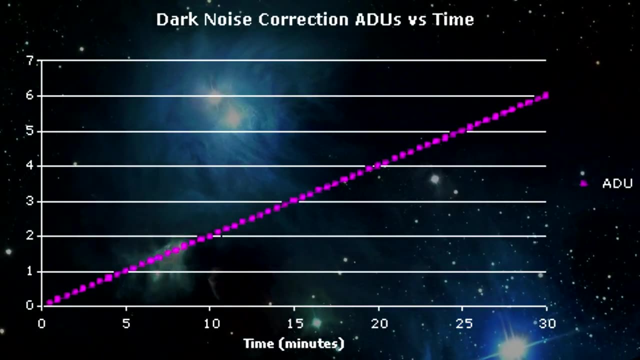 field frames. Dark signal refers to electrons that are generated in the absence of light as a result of thermal noise. These thermal electrons create hot pixels which increase in intensity over the exposure duration. Dark frames are images taken with the shutter closed, but for some period of time. usually. 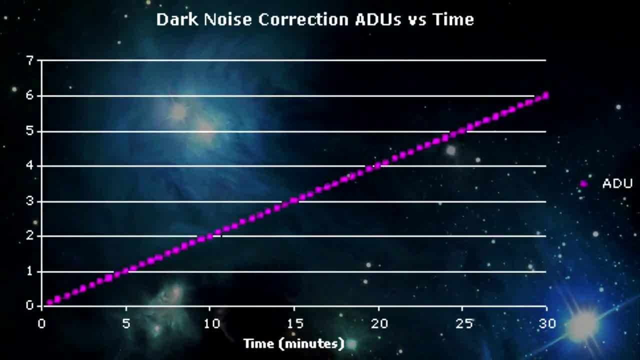 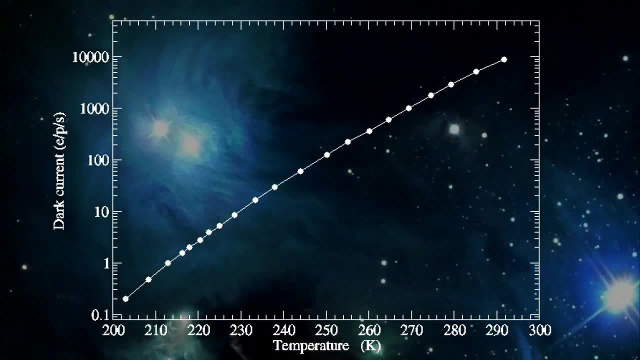 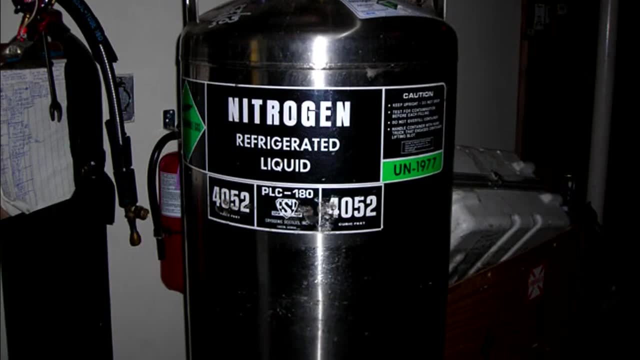 1,040 degrees. Unlike the standard face recognition of light, the Bias image is used with the shutter closed. Dark, subtle light changes the light. The Bias image of the picture is usually tantamount to the temperature of the image. The Bias image of the image is already a light, so we will correct it in aculus. 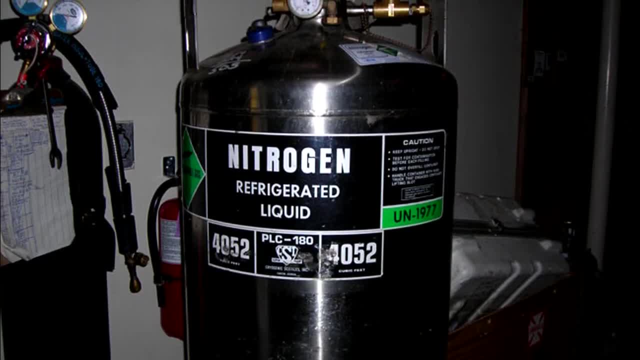 The effect of the Bias image is greatly reduced by cooling the CCD. Cooling the CCD from room temperature to minus 25 degrees will reduce the dark current by more than 100 times. Astronomical CCDs typically operate at temperatures below minus 70 degrees. Therefore, the effects of dark current in the images used in this tutorial are negligible. The Bias image is the result of the Bias channel. It will have aективism and magnetic properties for the entire image. The Bias image is always the effect of a dark channel. 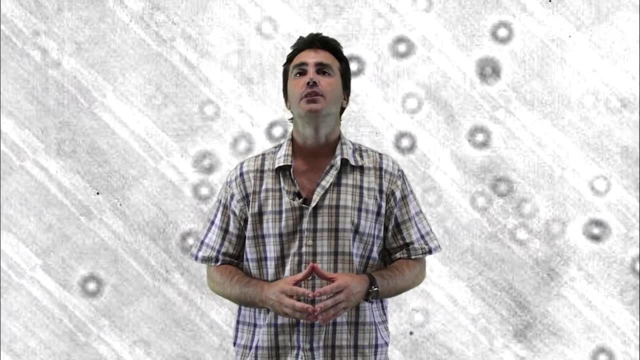 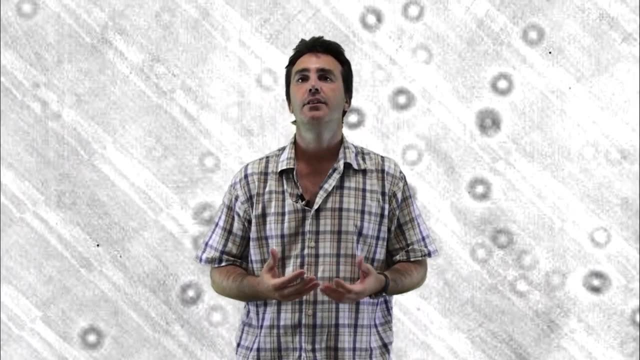 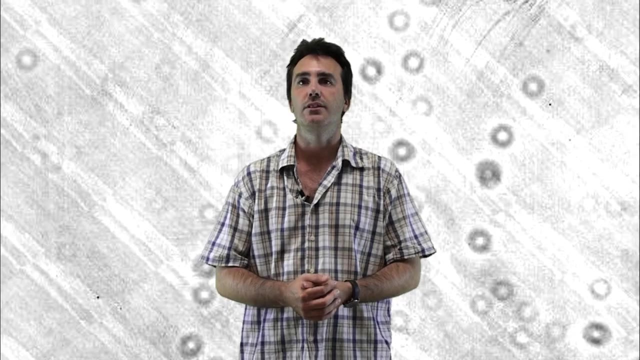 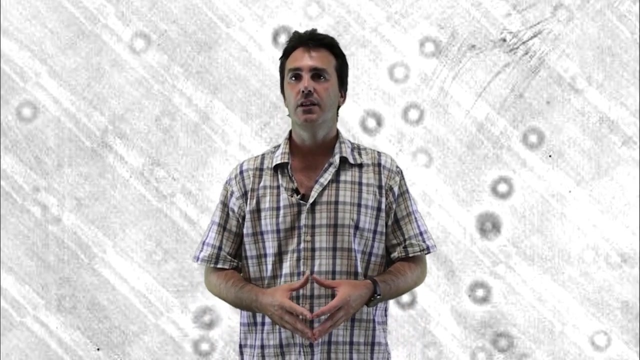 Today's CCDs are made to exacting standards. Still they are not perfect. Each pixel on the CCD may have a different sensitivity to incoming photons due to small variations in individual pixel dimensions and quantum efficiency. For precision photometry it is necessary to calibrate such pixel-to-pixel variations, and this is the function of flat field. 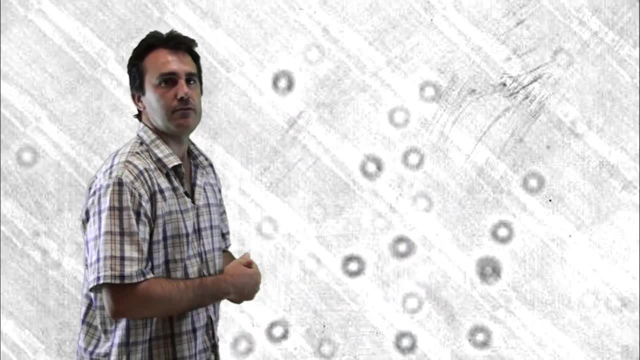 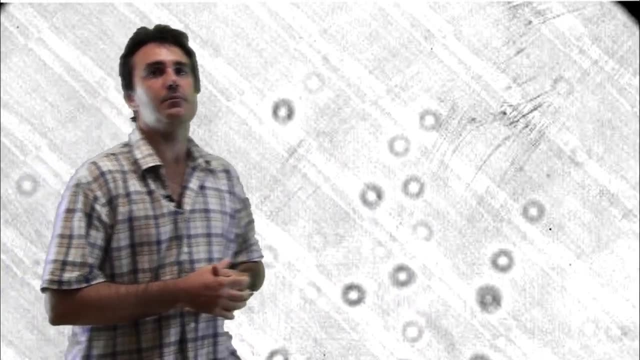 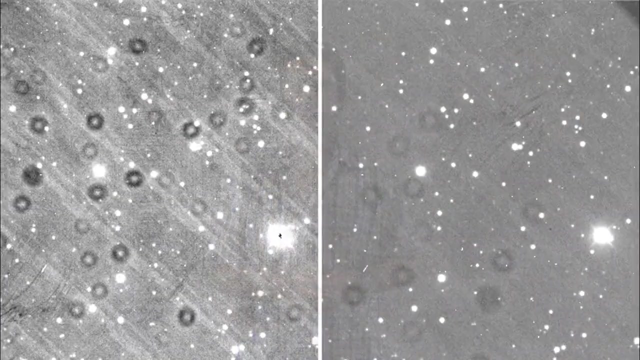 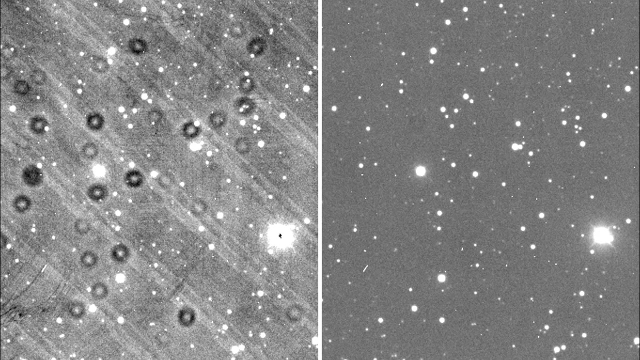 This image corresponds to a flat field frame. You can see dust, moats, some electronic structure and vignette in it. Flat field images are used to eliminate all these effects and other optical variations in the imaging system. On the left you see the raw image where all these artifacts are present and on the right the image after correction where all these artifacts have disappeared. 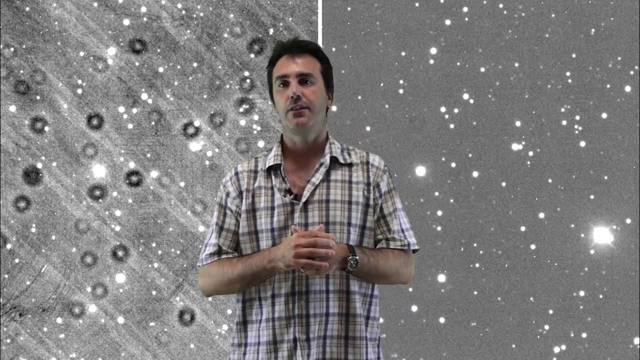 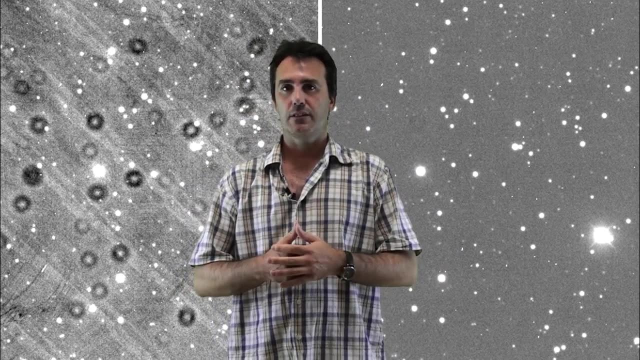 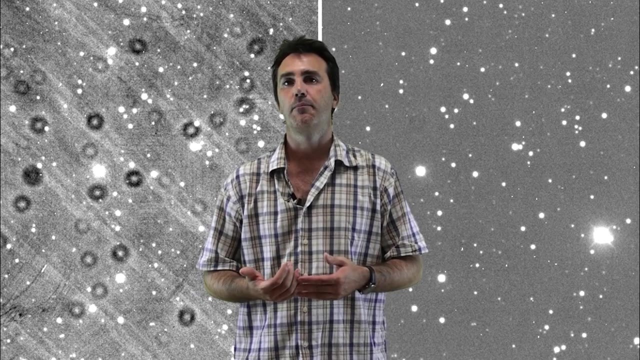 There are two important things to consider. There are two important differences with respect to bias and dark frames. First, unlike bias and dark correction, which are additive effects, flat fielding is a multiplicative effect, So the data have to be divided by the flat field. 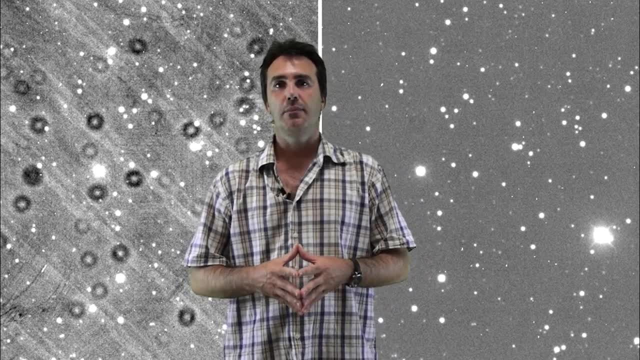 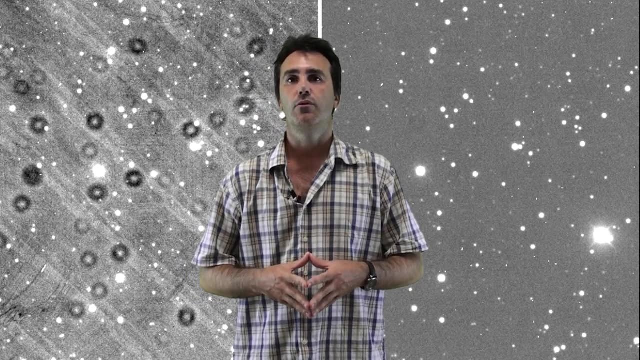 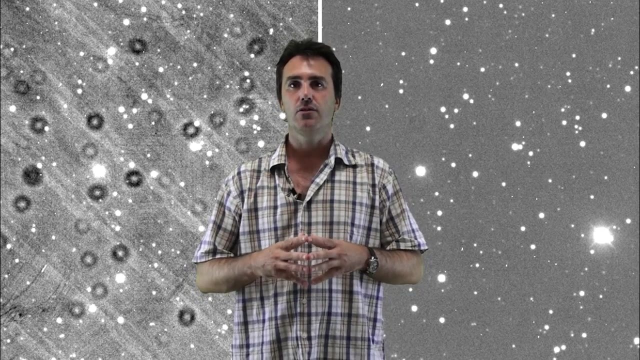 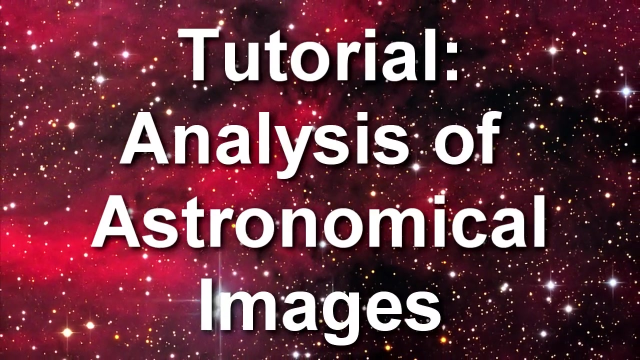 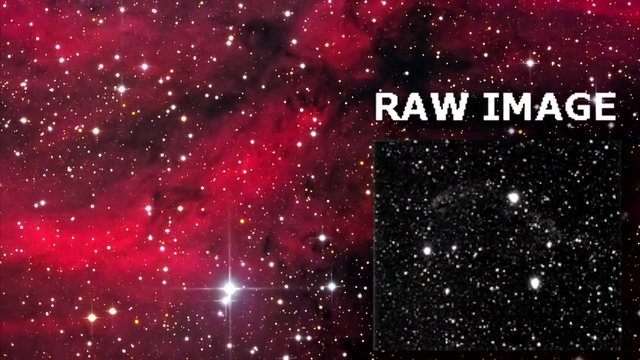 Second, the response of a pixel depends on the wavelength of the incoming radiation. Therefore, the flat field correction has to be performed for each filter separately. Now you are ready to follow the tutorial. Analysis of Astronomical Images. We are now going to show, step by step, how to remove the instrumental effects from a raw CCD image. 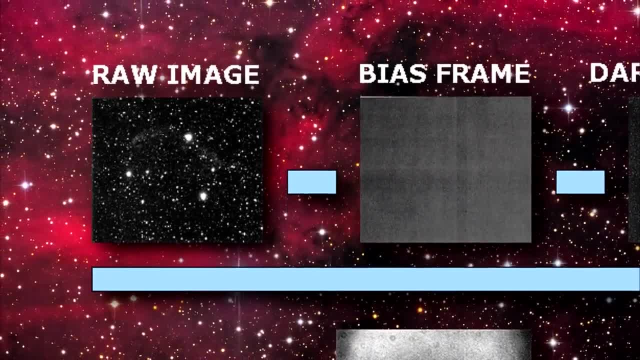 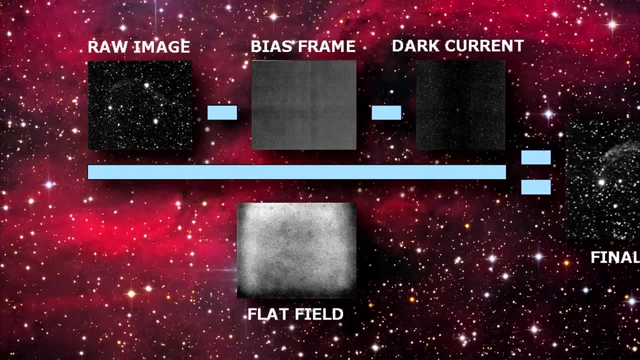 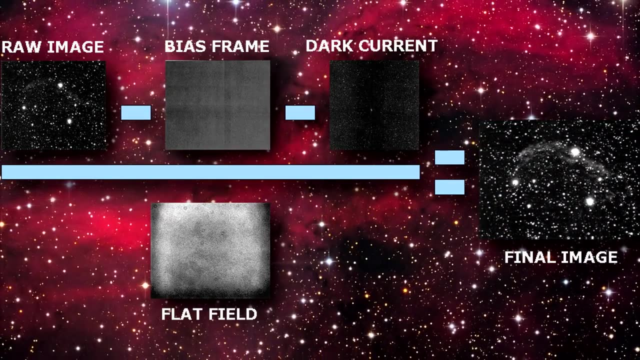 You will learn how to subtract the bias level, how to correct for pixel-to-pixel variation. that is flat fielding. However, we will assume that the dark current is negligible. You will also learn how to estimate the scene of an image. I will assume that you have installed the iDRAF and DS9 software packages in your computer. 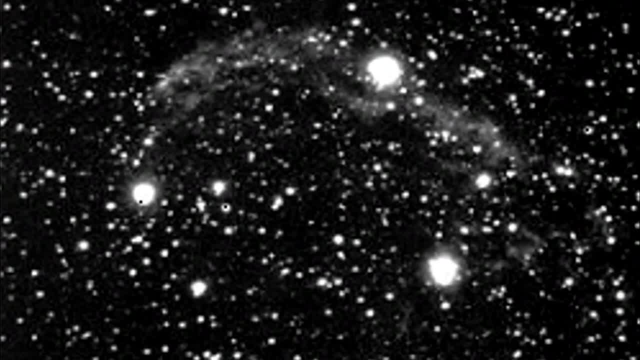 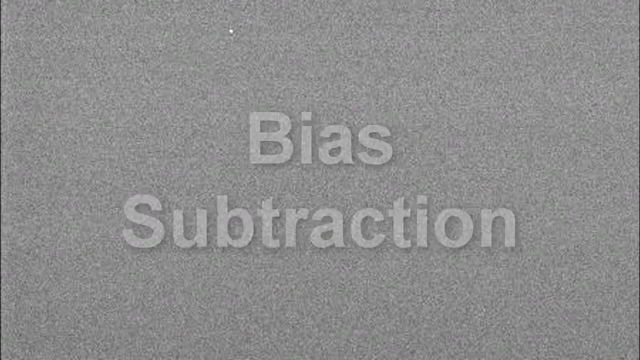 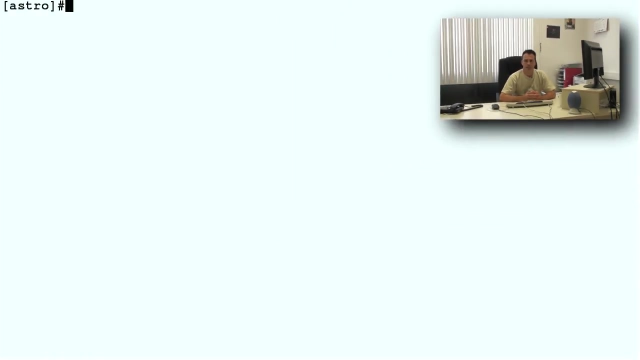 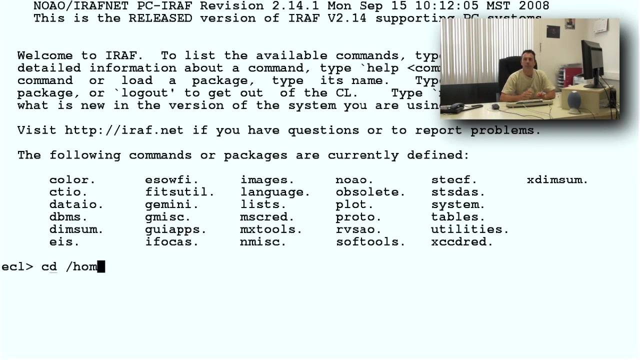 and you have run mkiDRAF. to create a logincl file, You must have downloaded and uncompressed the data file. The data file is calibrationtar. Our starting point is the directory where the file logincl is located. First we start up iDRAF by typing ecl. 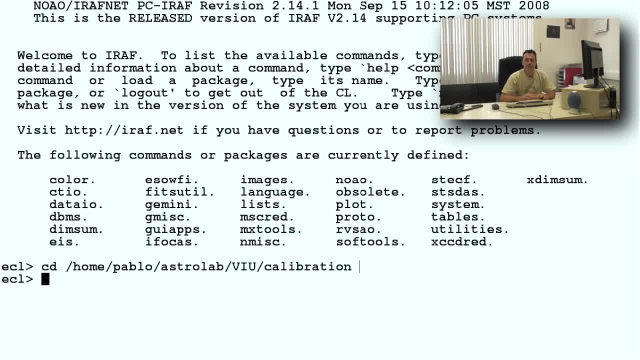 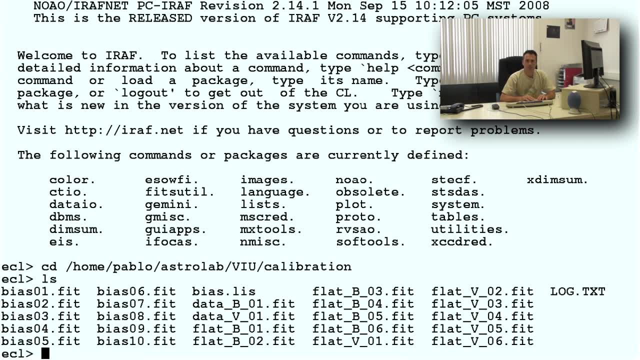 Then we go to the directory where the data are stored. As you can see, there are several bias frames, several flat field frames taken through different filters and a couple of data files. There is also a file called logtxt that contains information about the observation. 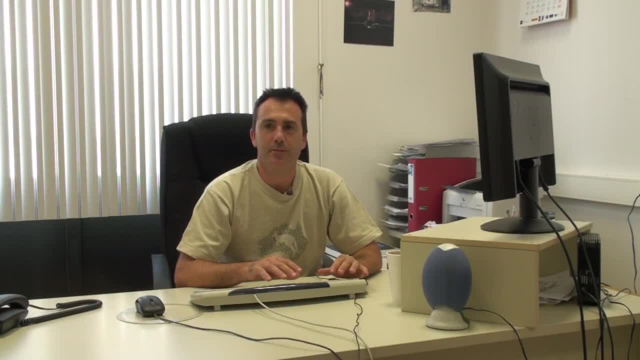 Bias frames are zero-second exposures obtained with the shutter closed. Therefore, we do not expect to see any star in a bias frame. The bias level is different for different CCD cameras. However, the bias value in a CCD image is usually constant with time, except for statistical fluctuations. 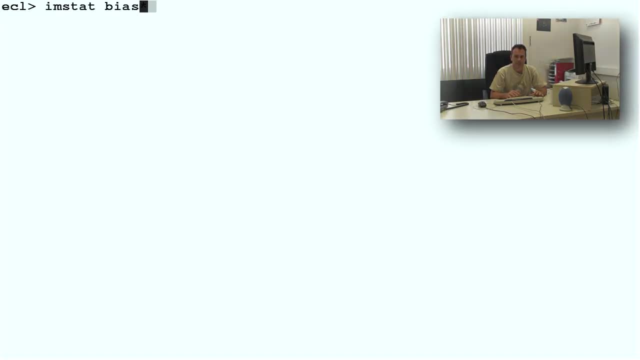 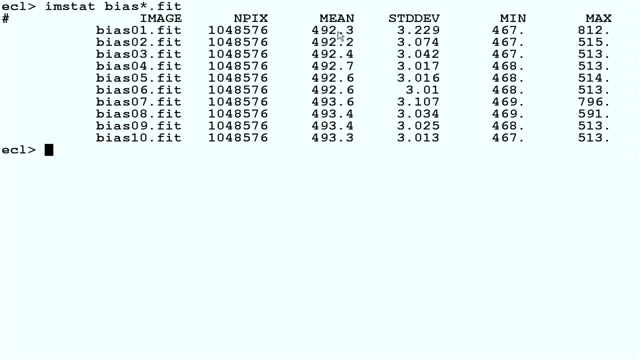 With the iDRAF task, imstat, we can print out statistical information of the image. As you can see, the mean value for each bias frame is 0.1.. Finally, the mean value for each bias frame does not change much. 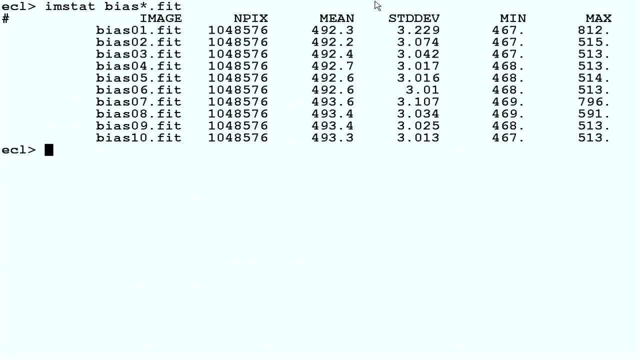 These bias frames were taken throughout the whole night. Indeed, the bias level remains pretty constant. To create a mean bias frame, we put together in one file the name of all bias images. This is done with the iDRAF task files. 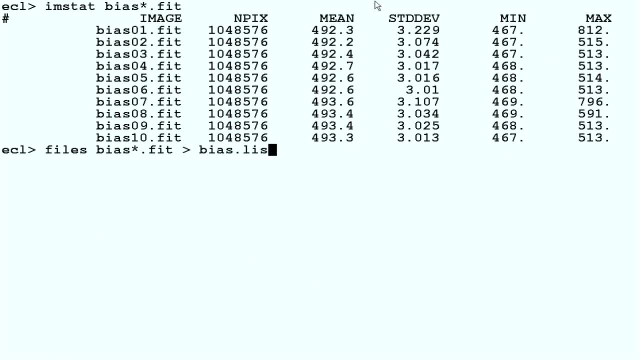 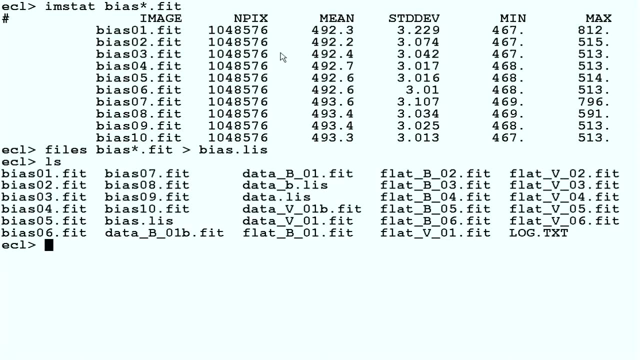 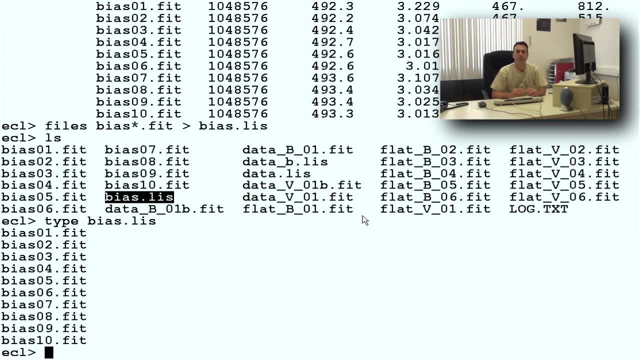 This task lists all files matching the given template. The larger than symbol redirects the output to a file. In this case the file name is biasthis. With the task type we can view the contents of the file. Now we are ready to combine all bias images to produce one mean bias frame. 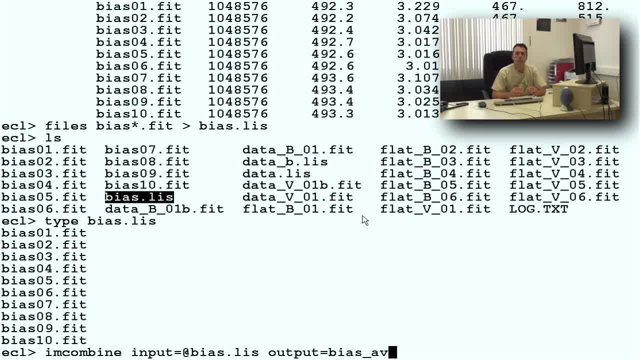 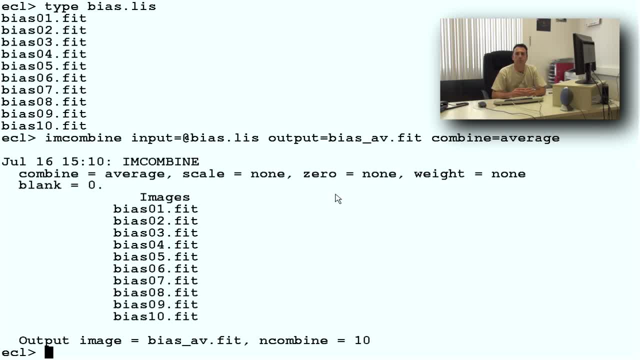 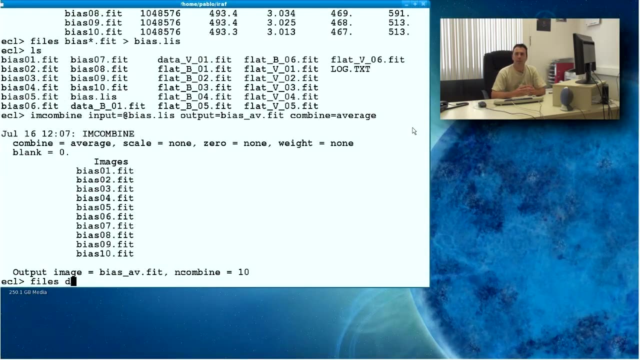 The iDRAF command that allows us to do this is imcombine. The output is the file bias-appfit. Once we have the mean bias frame, we can proceed to subtract it from the data frames As before. create a file with the name of all the data frames. 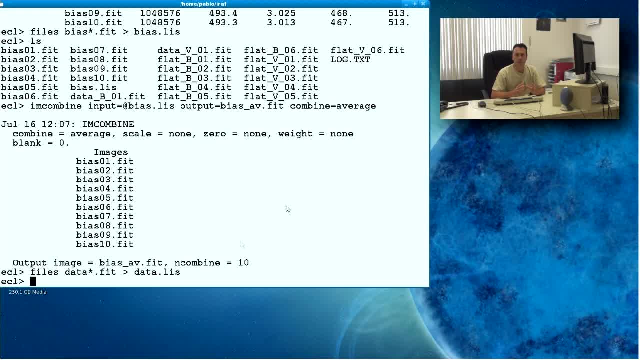 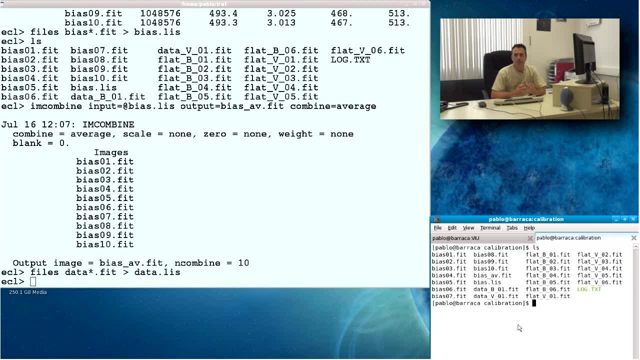 For example, datalist, One file name in each row And use this file as input. The output can be the same datalist file, but the images will be overwritten If you want to give a different name to the bias-subtracted images. 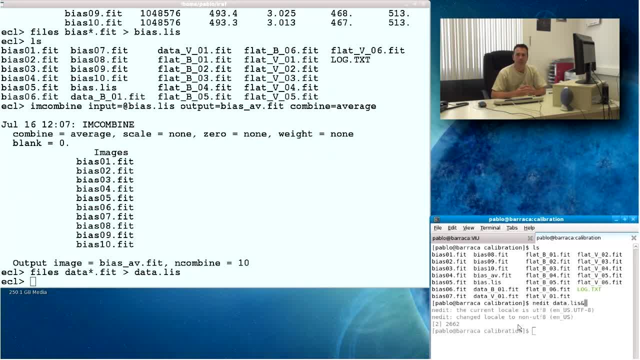 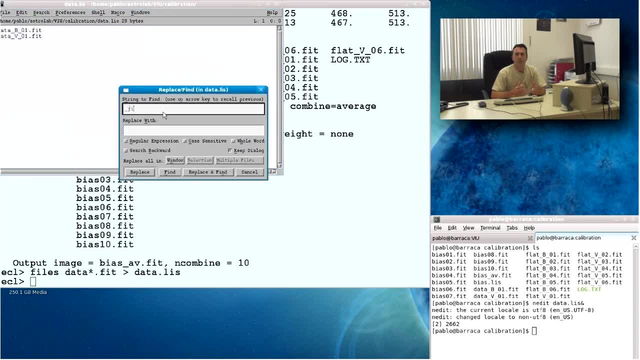 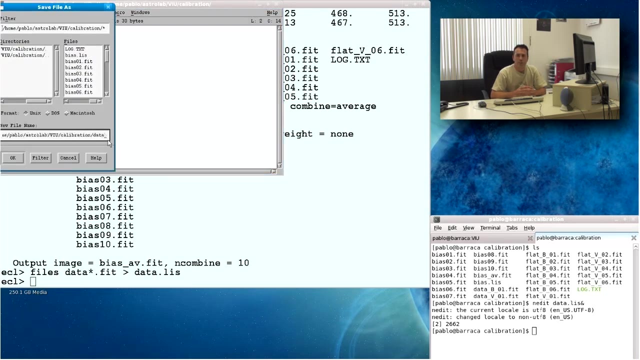 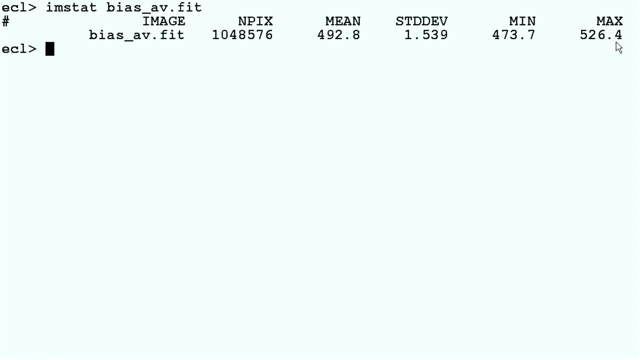 then change the file names inside the datalist file and give it as output. You can change the names by editing the file datalist using your favorite editor And editlist. Don't forget to save the new file with a different name. The mean bias level is 492.8 ADU or counts. 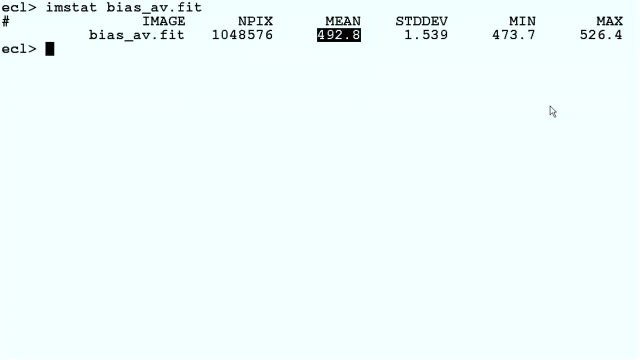 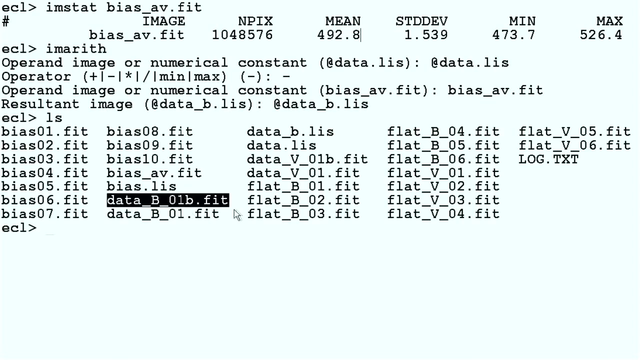 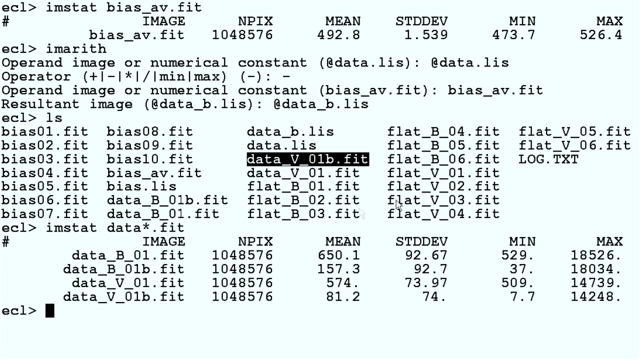 The subtraction of this bias level is done with the task imarith. The input is the datalist file And the output the datalist file. This creates the files datab01b and datav01b. As you can see the difference in counts between the data files. 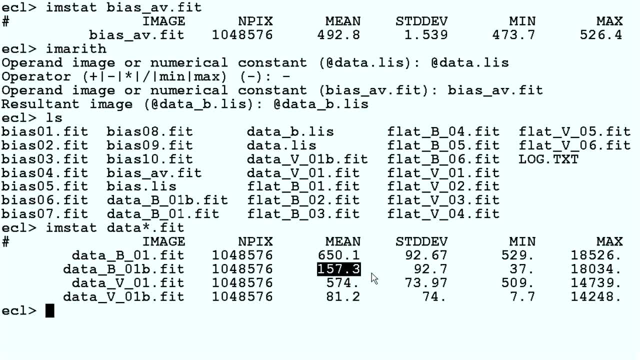 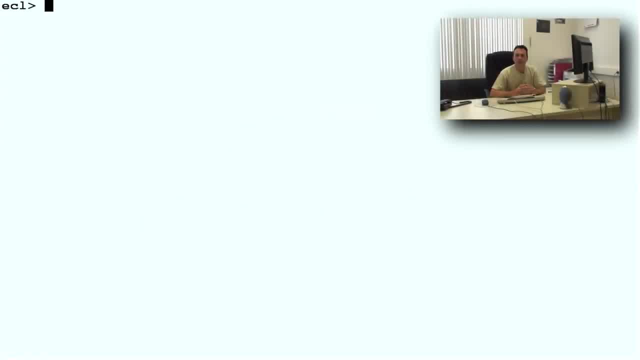 before and after. the bias subtraction is the mean bias level. Each pixel on the CCD camera may have a different value. Each pixel on the CCD camera may have a different sensitivity to incoming photons due to small variations in individual pixel dimensions and quantum efficiency. For precision photometry it is necessary to calibrate such pixel-to-pixel variations. 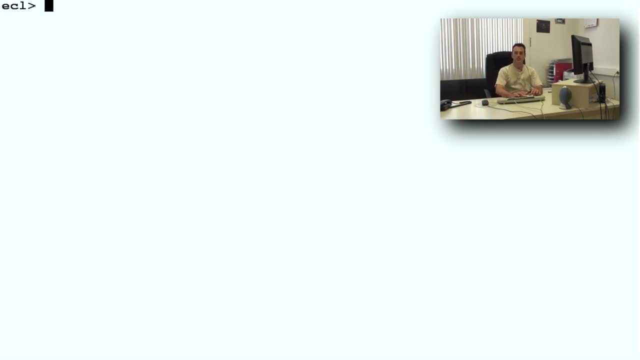 and this is the function of flat fielding. Flat field images are also used to eliminate the effects of vignetting, dust modes and other optical variations in the imaging system. The steps to perform the flat field correction are: 1. Normalize the average count of each flat to 1.. 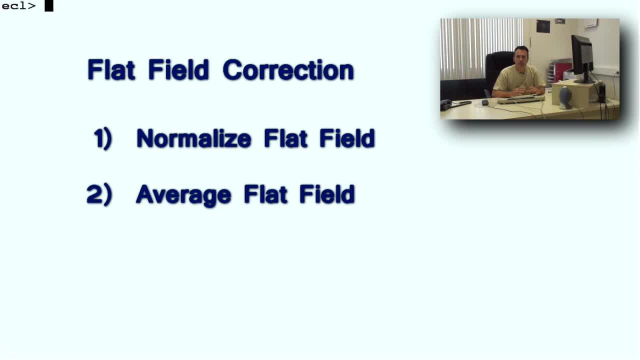 2. Obtain one average flat field frame for each filter. 3. Divide the data frames by the average flat field. The normalization can be done with the task Normalize in the iDraft package. knowhow in red generic. So let's load these packages. 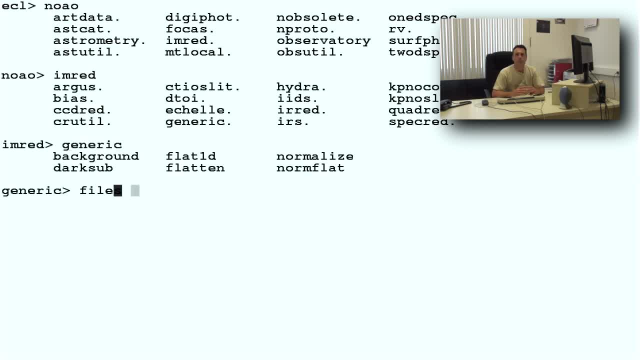 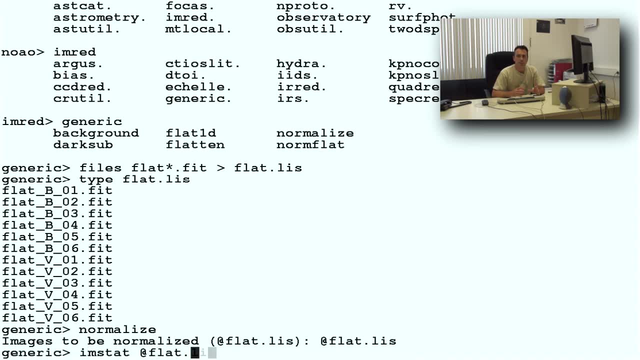 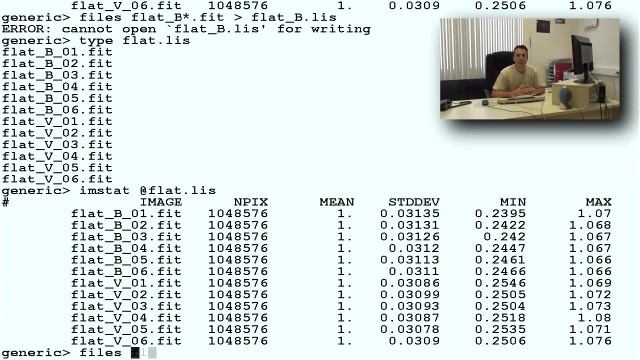 Now we create the list of flats. Let's check that the mean is 1.. Let's check that the mean is 1.. The response of a pixel depends on the wavelength of the incoming radiation. Therefore, the flat field correction has to be done for each filter. 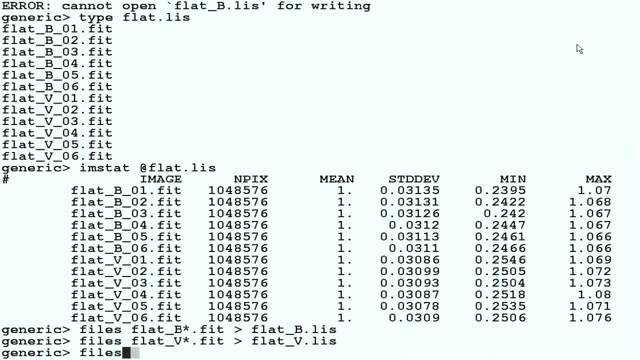 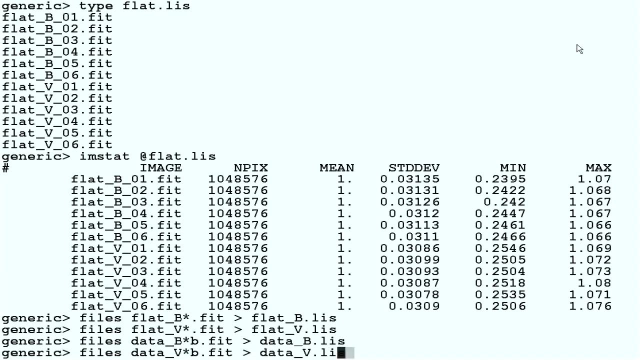 So we create lists of flats and data frames for each filter separately. Remember to use the data frames for which the bias level has been subtracted. Now we can proceed and obtain one average flat field for each filter. Again, this is done with the iDraft task mcombine. 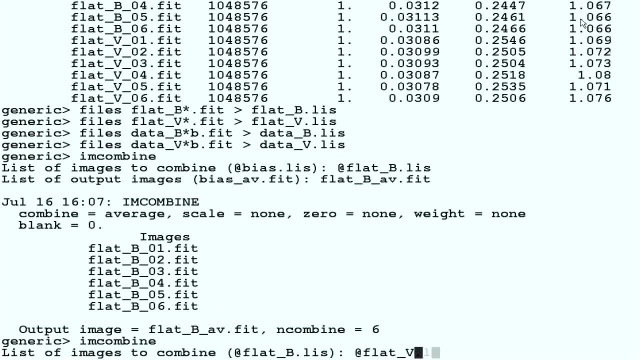 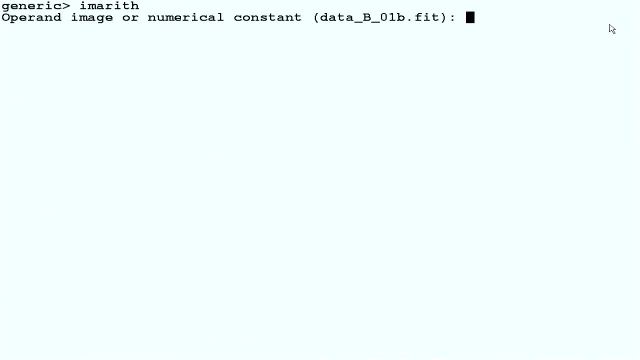 Finally, we divide the data frames by the average flat field with the task imarith. If you do not want to overwrite your data files, create another list for the output of imarith. For example, we will add the suffix f. In this case, we have only one file in each filter. 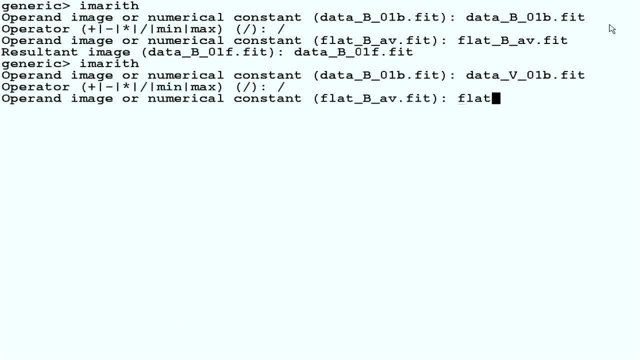 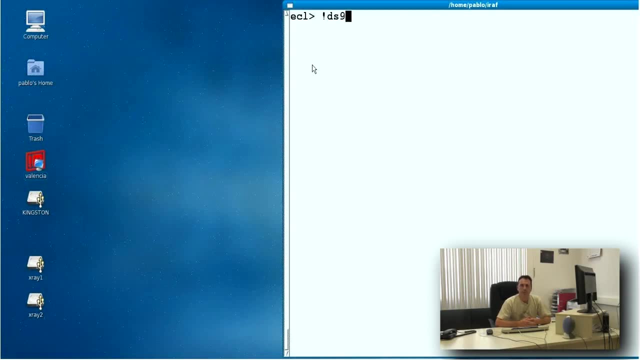 So we can apply imarith directly to the data frame. If we had many data files, we would make use of the list. Let's summarize the whole procedure by displaying some representative images. Let's summarize the whole procedure by displaying some representative images. 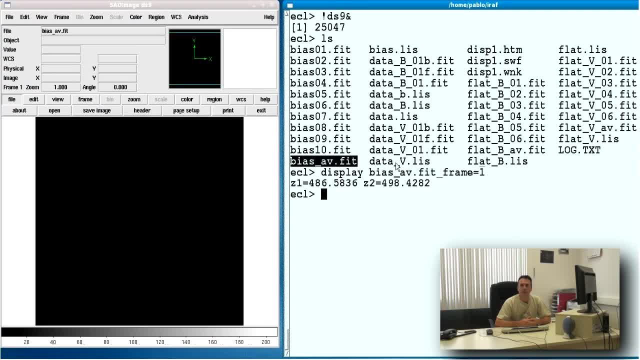 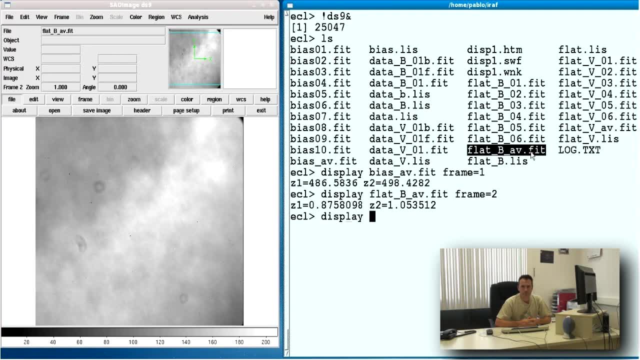 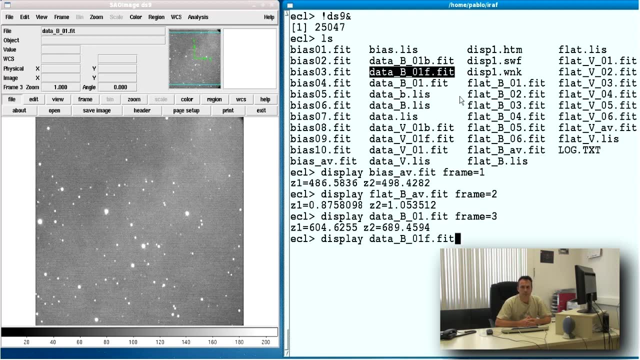 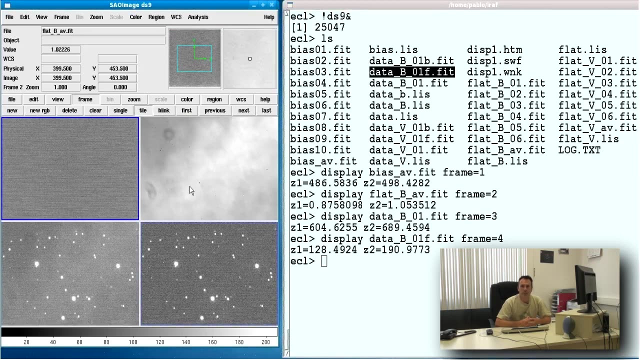 First, the mean bias level frame. Second, the mean flat field frame for the B filter. Third, the raw data frame in the B filter without any correction. And finally, the data frame in the B filter after subtracting the bias level and dividing by the flat field. 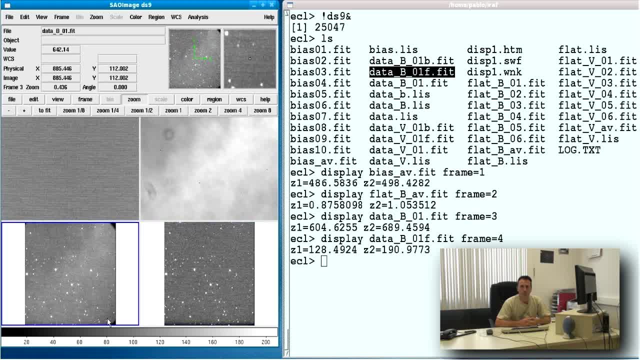 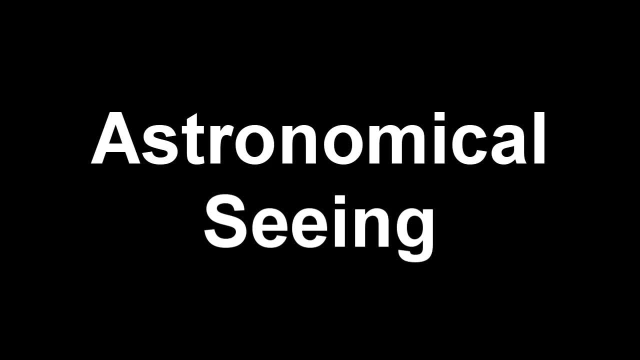 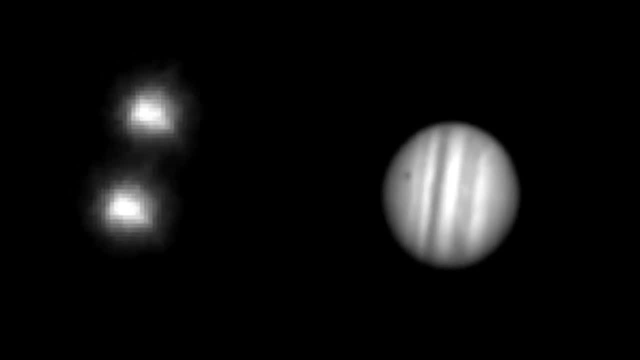 Note how the vignetting and the homogeneous illumination effect do not appear in the final image. Astronomical seeing refers to the blurring and twinkling of astronomical objects, such as stars, caused by turbulence in the Earth's atmosphere. Stars are so far away that for all practical purposes, they can be considered as point sources. 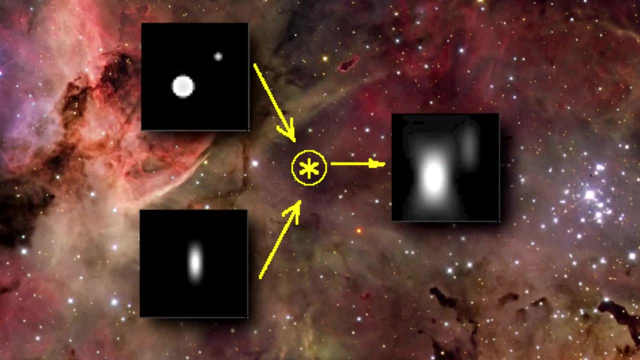 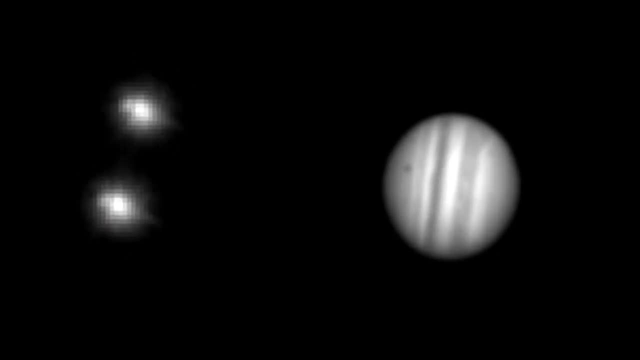 Although the source may be a point, the image of a star on your camera is not Astronomical. seeing describes how much the Earth's atmosphere perturbs the images of stars as seen through a telescope. Therefore, it describes the conditions of the night sky and how suitable it is for astronomical observing. 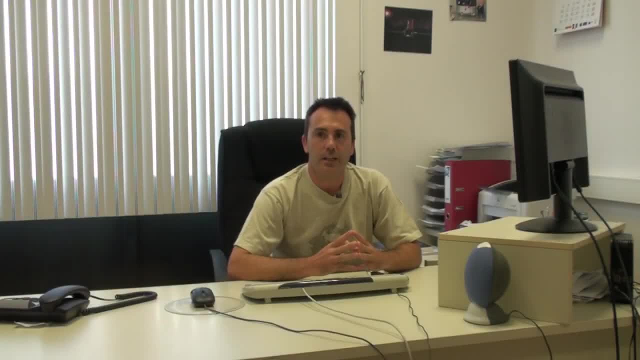 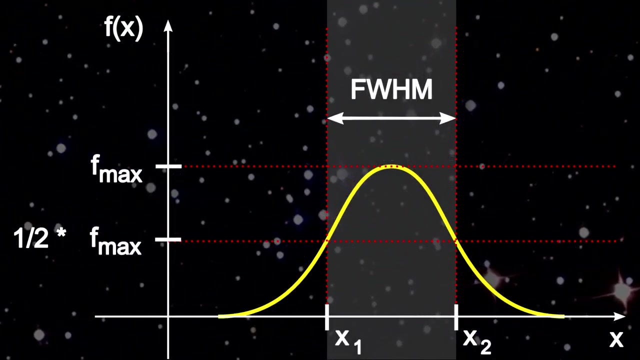 Therefore, it describes the conditions of the night sky and how suitable it is for astronomical observing. It is comprised of two parts. through the telescope and the opacity of the atmosphere, that is how much stuff is floating around in the air. The most common way to estimate the scene is to 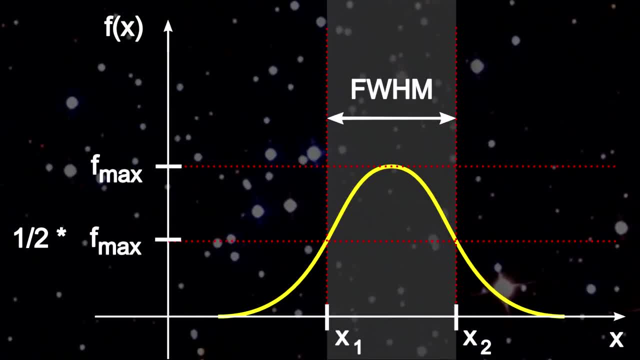 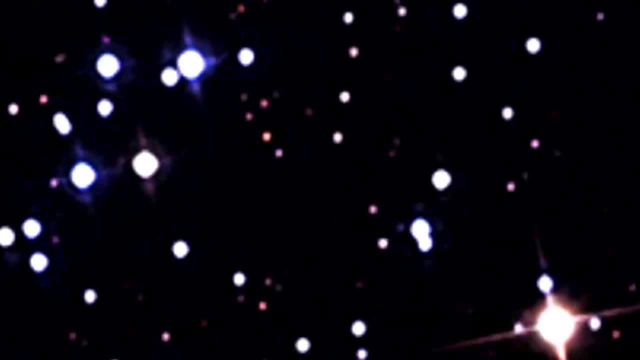 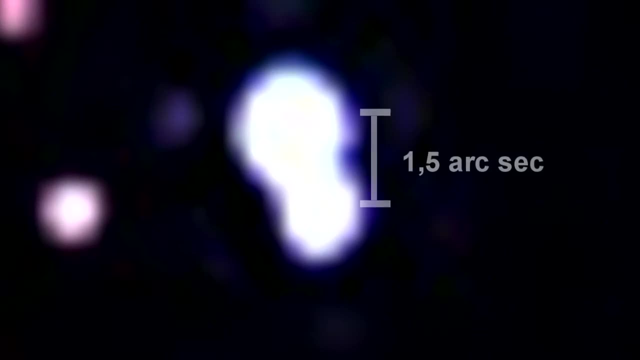 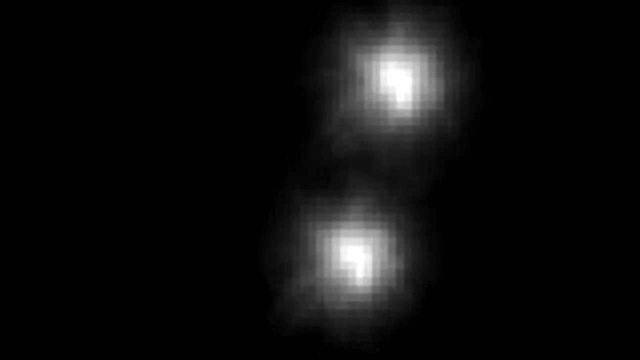 measure the diameter technically the full width at half maximum of the point spread function. The point spread function, diameter or scene is a reference to the best possible angular resolution which can be achieved by an optical telescope in a long photographic exposure and corresponds to the diameter of the fuzzy blob seen when observing a point-like star through the. 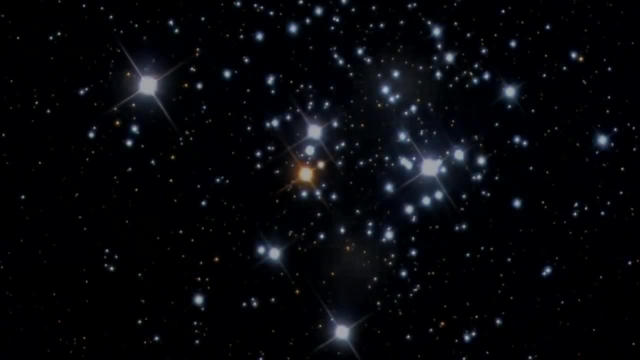 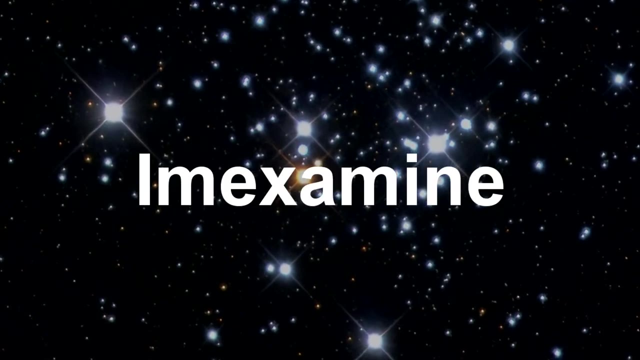 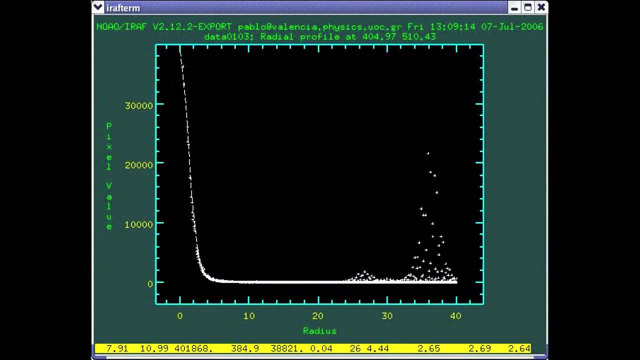 atmosphere. The giraff task imexamine is often used for the estimation of the scene by performing a Gaussian fit to the radial profile of a star. The full width at half maximum of the radial profile can give a good approximation to the scene. for well sampled images, The radial 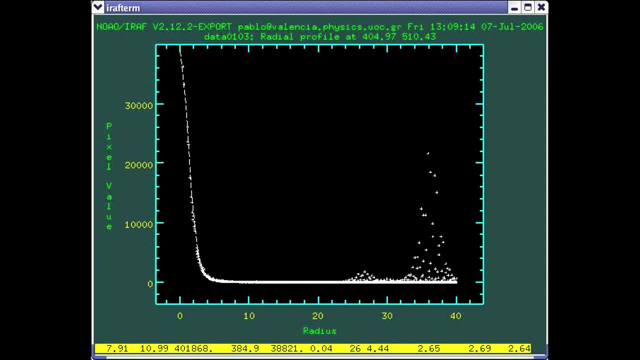 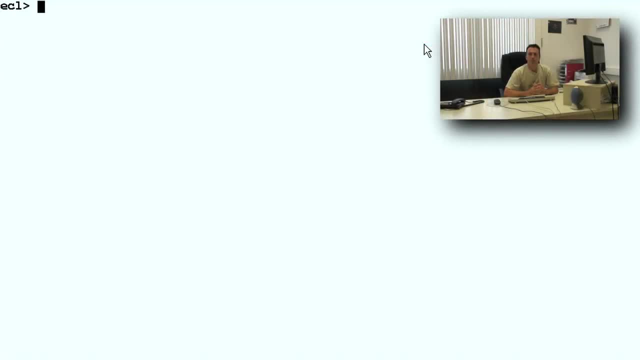 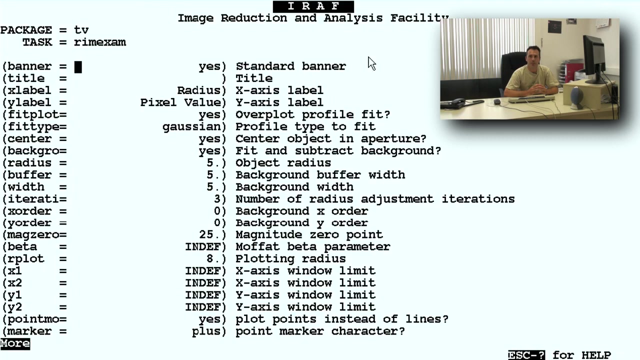 profile is the variation of the flux as we move out from the center of the star. First let's check the plotting radius. If needed, set it to a value of about 18 to 20 pixels. We do this by editing the parameter file rimexam and changing the value of the plotting radius To exit. type ctrl D. 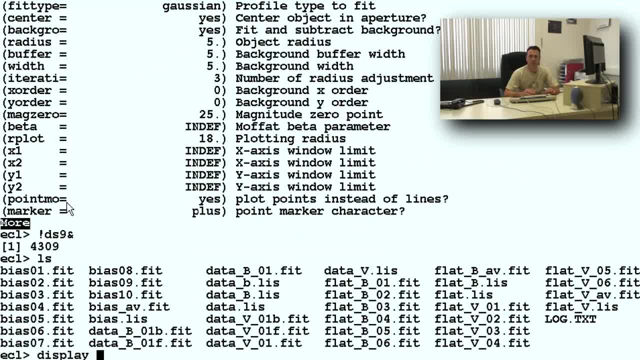 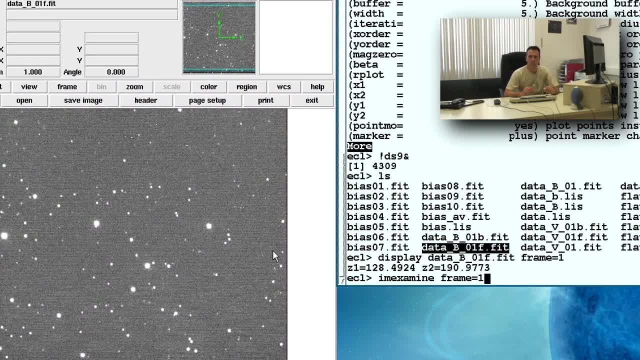 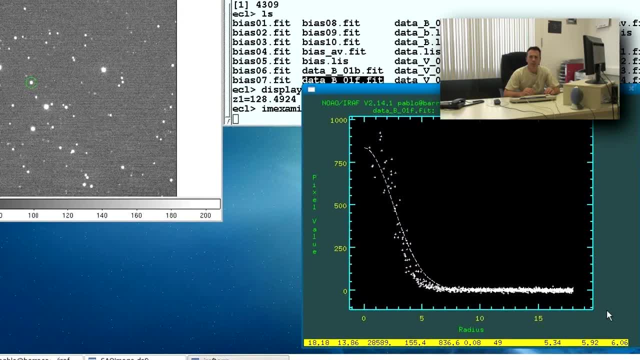 Let's display a bio-subtracted and flat-field corrected image. Run the task, imexamine, Move to an isolated star and press the key R. The three red- most values- give the full width at half maximum of the radial profile. We will take this value as a measurement of the scene. Move to another star and press R.